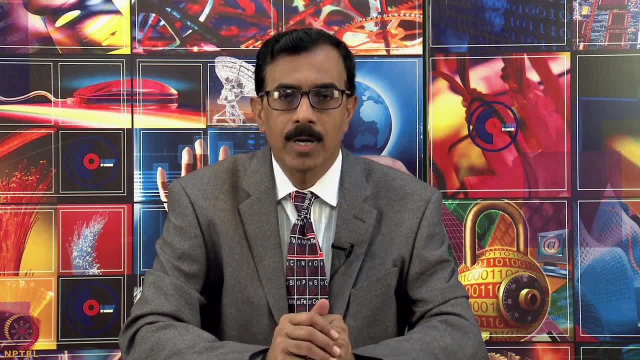 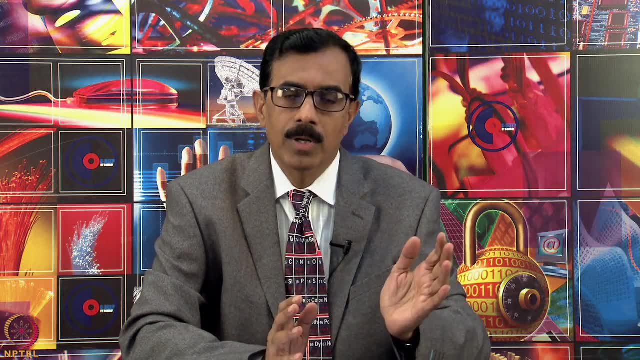 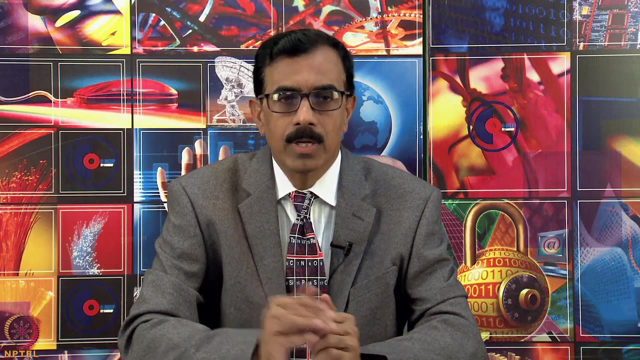 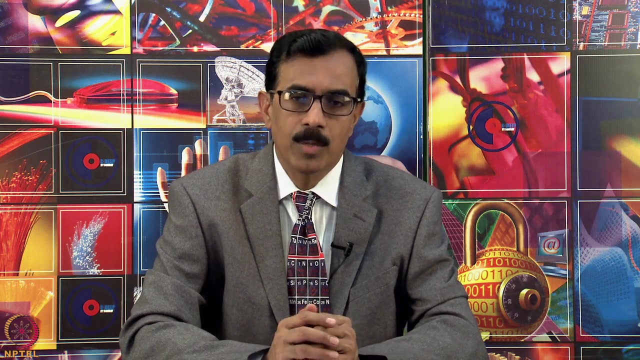 is NS2NP6. that means octet is completed and in fact most of the elements in the periodic table which come left in the groups have a tendency to have the electronic configurations of noble gases and this we call it as octet in case of S and P block elements, because 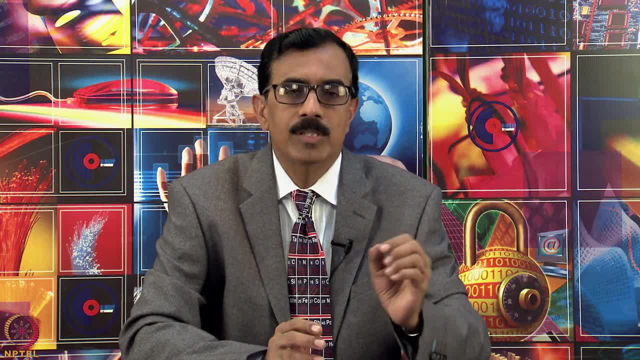 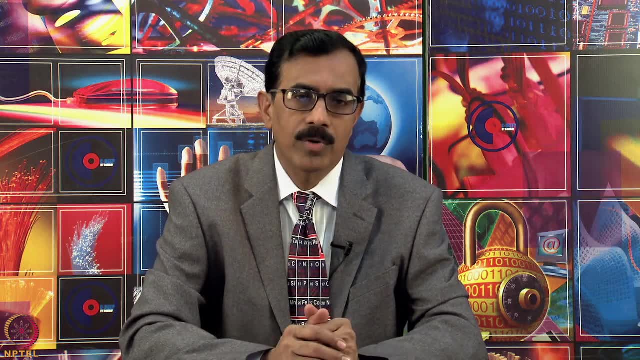 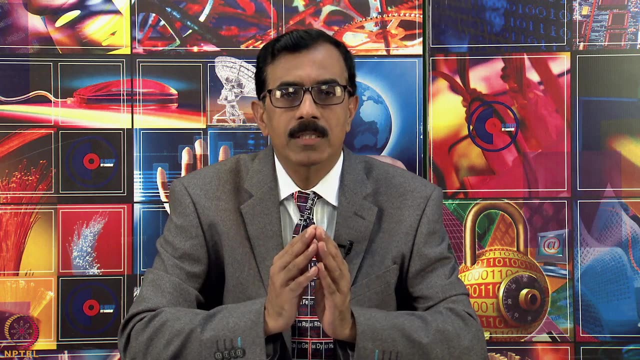 all of them have a tendency to have S2P6 or NS2NP6 electronic configuration. Noble gases or inert gases have that electronic configuration and, as a result, they are very, very important and very stable, having very high ionization energy. So the noble gases have also been 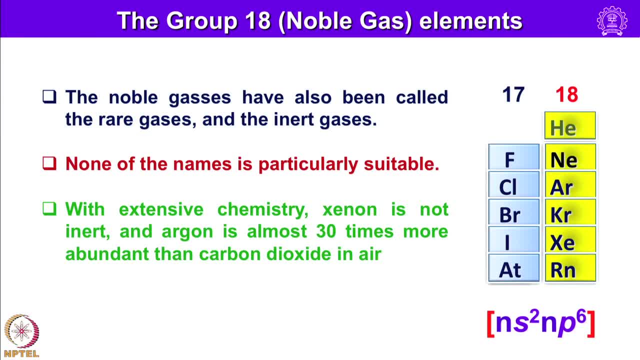 called as rare gases and, as we know, they are also called as inert gases. Of course, now, none of the names it appears are particularly suitable With extensive chemistry. xenon is not inert, and argon is almost 30 times more abundant than carbon dioxide in air. Try to know little bit more about this group 18 elements. the greater reactivity of xenon compounds compared to the other group 18 elements. Of course, only other element that known to react is krypton. So xenon shows greater reactivity and the stability of xenon compounds containing. electro negative elements such as oxygen and fluorine, The reactivity of noble gas fluorides as fluoride ion donors and acceptors. In fact, it is known that inert gases are group 18 elements possess extremely high ionization energy. As a result, initially it was assumed that they are not suitable for making chemical compounds. The first xenon compound was synthesized in 1962. Since then the chemistry of xenon is quite extensive. The compounds of krypton have also been reported. The chemistry of main group gas compounds. 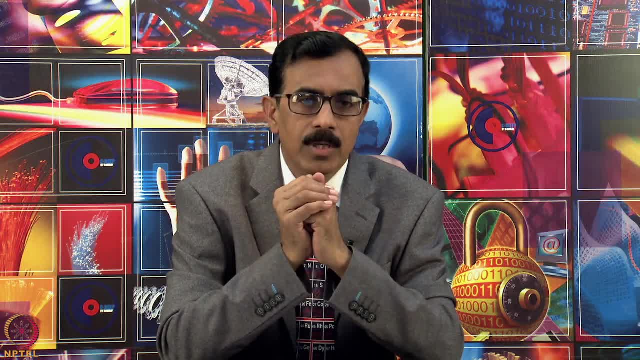 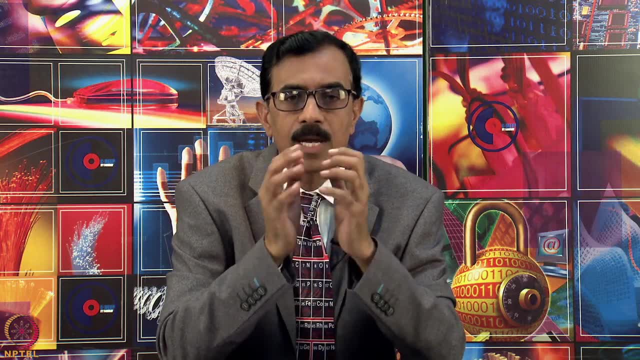 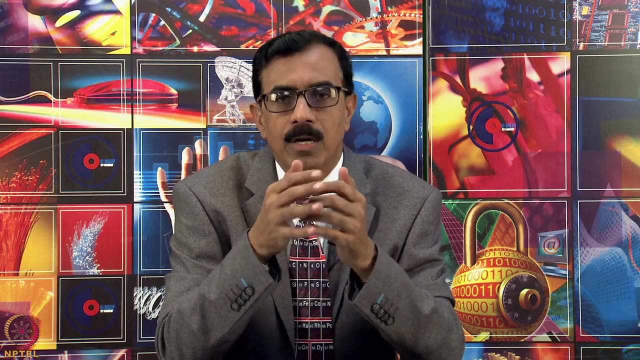 are analogous to those of heavier group 17 elements and VSEPR theory is a very powerful technique for nationalizing and predicting the shapes of many noble gas compounds which have relatively large number of electron pairs in the valence shell of the central atom. Noble gases have filled shells, that is, Ns to Np6, completely filled, having 8 electrons. So, in order to form chemical compounds, electrons must be promoted into the next shell. So, depending on the number of electrons promoted, compounds of the noble gases in earthen states plus 2,, plus 4,, plus 6 and plus 8 have all been synthesized. Just if you recall, the inter halogen compounds, group 17 elements show plus 1,, plus 3,, plus 4,, plus 5 and plus 7, apart from minus 1 earthen state, Whereas group 18 element shows plus 2, plus 4,, plus 6 and plus 8,. it is very simple if you just write the electronic configuration. 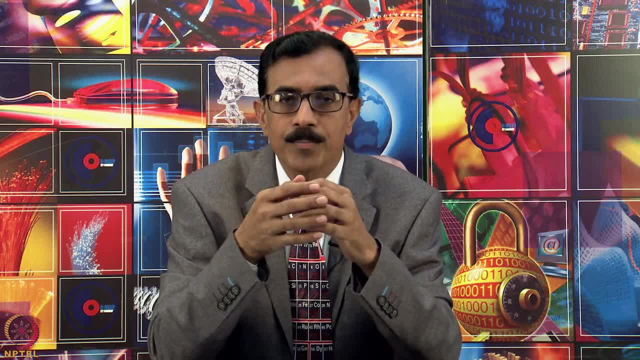 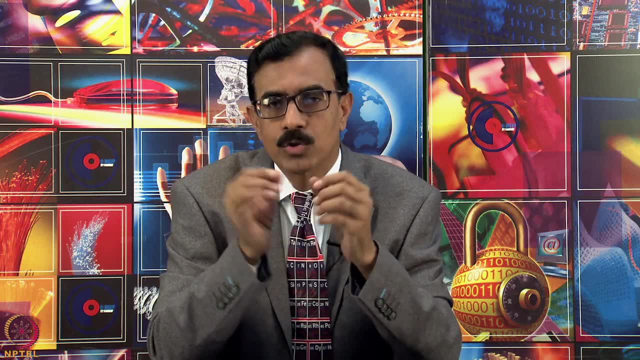 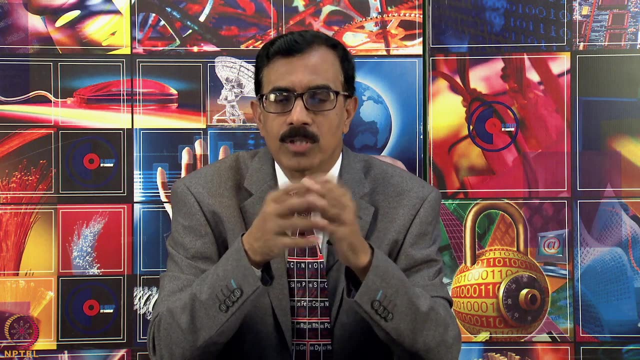 and just promote one electron at a time to the higher shell. you understand why. inert gases are group 18, elements shows plus 2, plus 4 and plus 6 and plus 6 and so on, Whereas inter halogen compounds are halogens and these are the normal gases. group 21 that means group. show plus 1, plus 3,, plus 5, plus 7. ok, It has to do with the electronic configuration, that is, the Ns2P5 and Ns2P6.. With increase in atomic size, the outer electrons are easily. removed and there is a decrease in first ionization energy. So, as a result, there are many xenon compounds, but a few for krypton, and none have been isolated so far. argon, The halogen compounds, halides, show minus 1, plus 1,, plus 3,, plus 5 and plus 7,, whereas 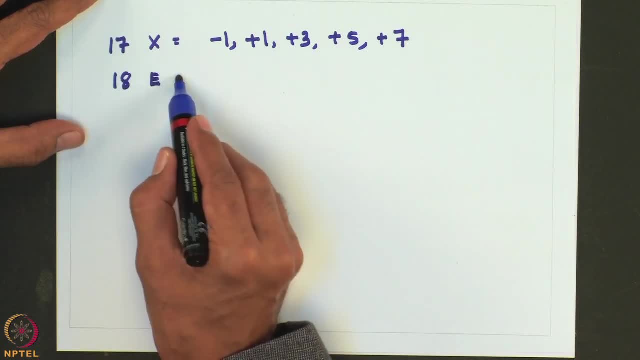 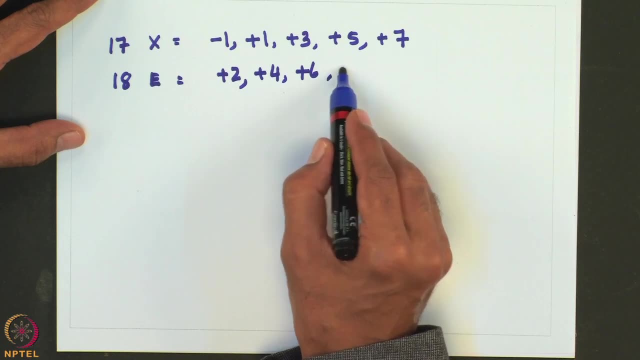 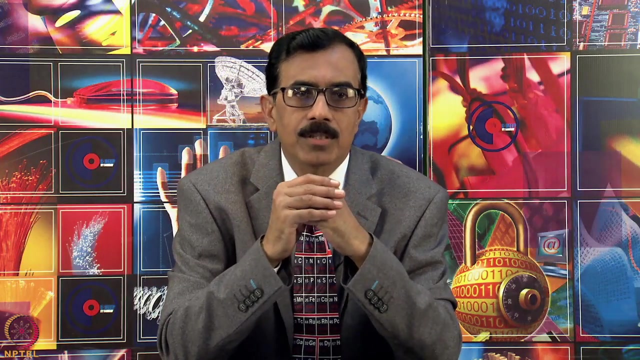 group 18 gases show plus 2,, plus 4,, plus 6 and also plus 8 oxidation states- I will come back to this one later- to be strong oxidizing agents and the fluorides are also very powerful fluorinating agents. The formation of anionic noble gas compounds, such as cesium neonide with electropositive metal is an intriguing possibility, though none has yet been isolated. Of course, this was reported in Journal of Chemical Education in 1988.. If you are curious to know the historical developments in noble gas chemistry, you can. 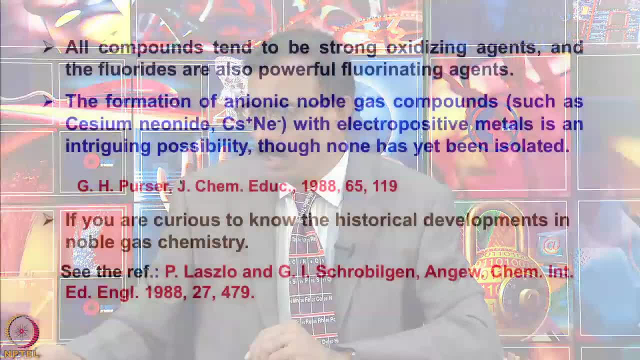 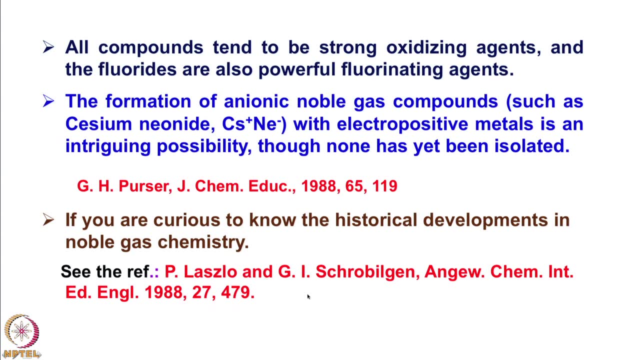 look into this article. here I have shown both the Journal of Chemical Education as well as the Angiochemi International Edition paper in which you can look into the information if you are more curious to know about some of these anionic nobles. So what is anionic noble gas compounds? 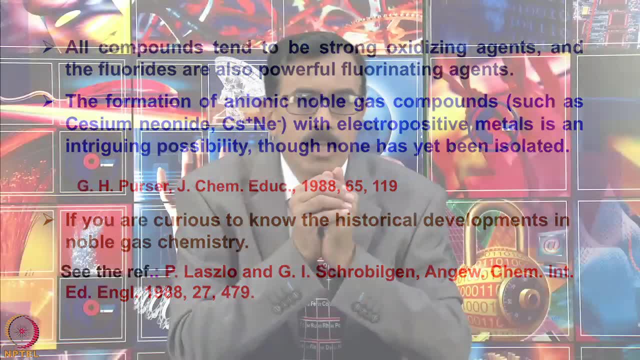 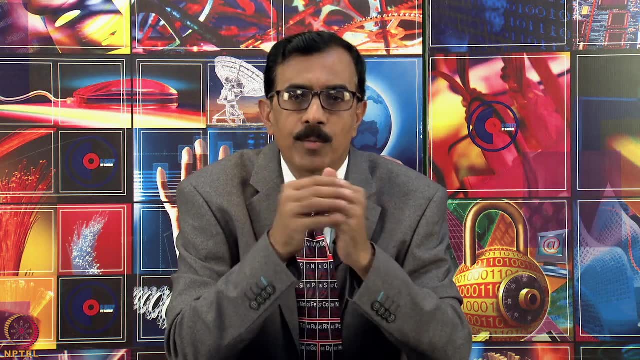 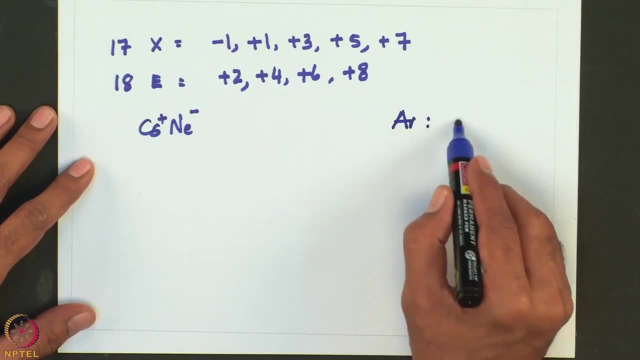 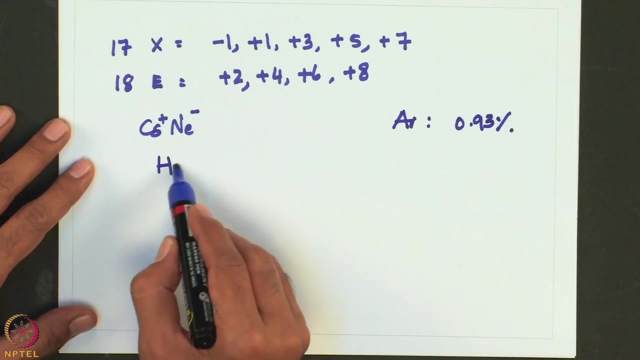 And also the historic development in noble gas chemistry. So all of the elements exist as highly unreactive monatomic gases with very low boiling points: Argon is the most abundant, comprising of 0.93 percent of the atmosphere, Helium, neon and krypton. 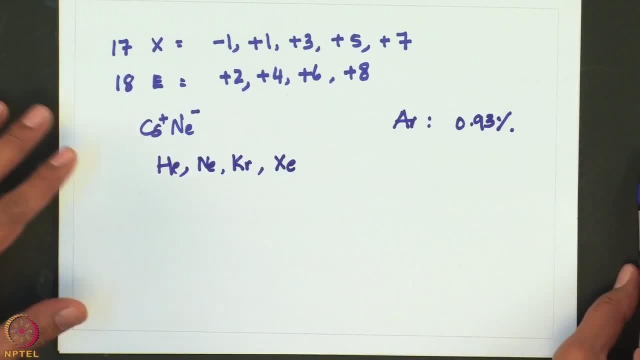 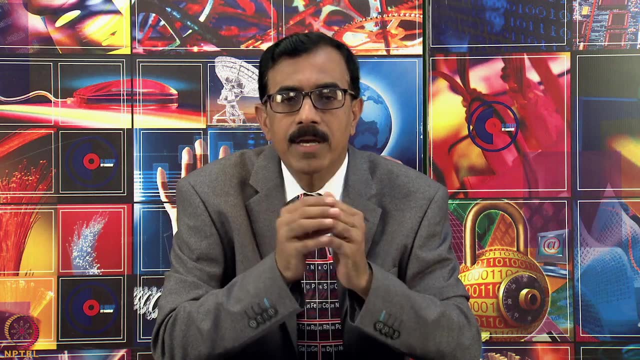 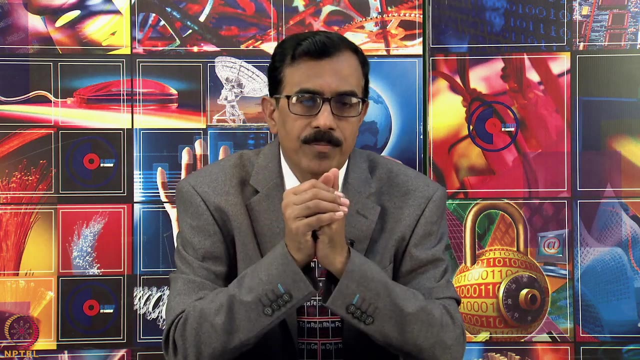 Ok and xenon are trace constituents of air. All isotopes of radon are radioactive and are formed naturally from the decay of heavy radio isotopes such as those of radium and uranium, Noble gas cloth threads. In 1920s and 1930s there was considerable interest in materials. 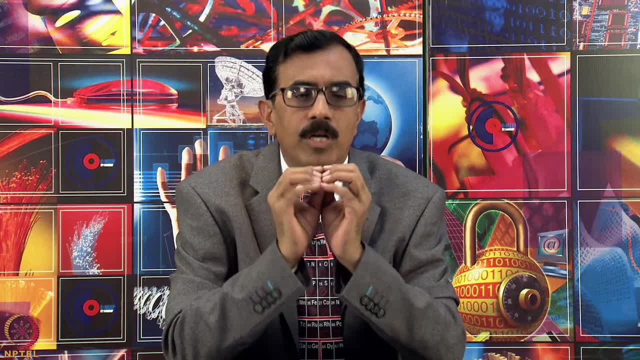 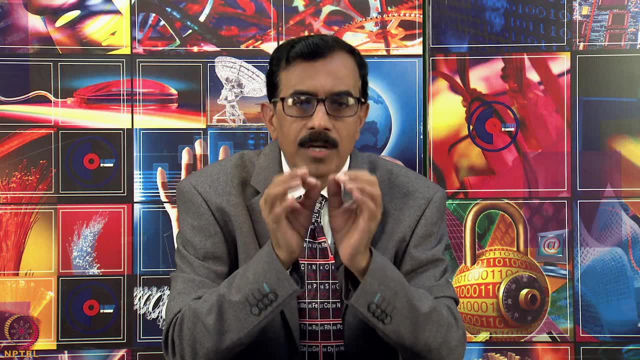 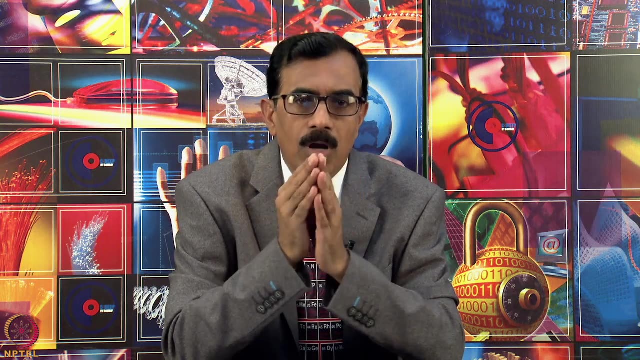 formed between noble gases, particularly those of argon, krypton and xenon, and strongly hydrogen bonding compounds such as water and polyphenols. Later it was shown that they are not actually chemical compounds, but they are inclusion compounds known as cloth threads, where the gas atoms occupy voids in the hydrogen bonded lattice of the host compound when the host is crystallized under noble gas atmosphere. For example, you take water or polyphenols and crystallize under a positive pressure. Under pressure of noble gases one can get inclusive compounds or noble gas cloth threads. 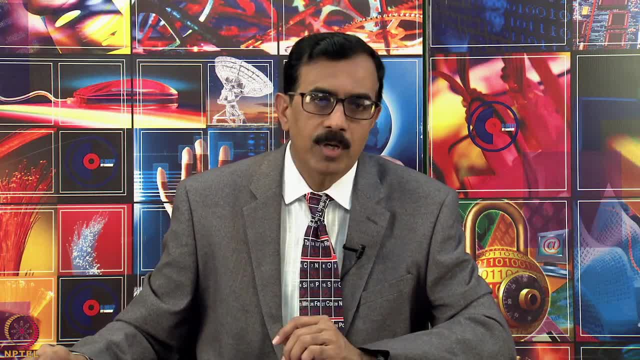 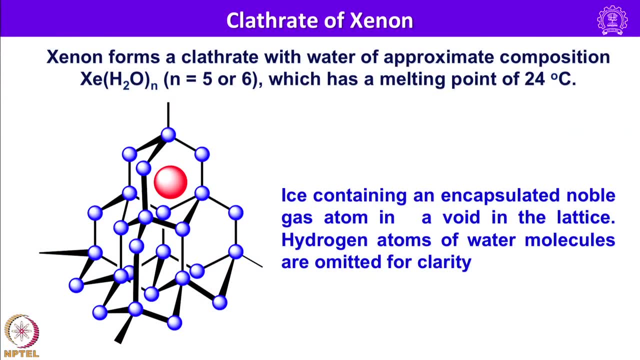 They are not actually the compounds with a chemical bond. So for example I have shown here: xenon forms a cloth thread with water of approximate composition Xe H2O n times, that is, n equals 5 or 6, which has a melting point of 24 degree centigrade. So ice containing 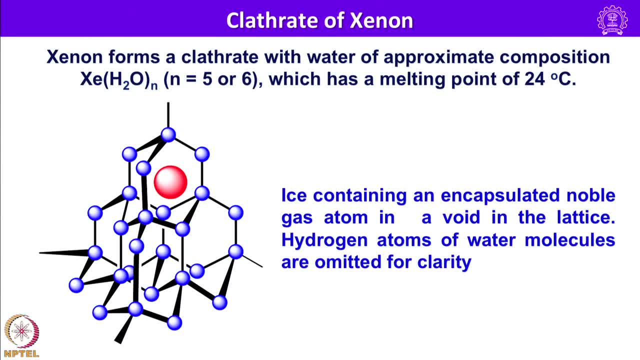 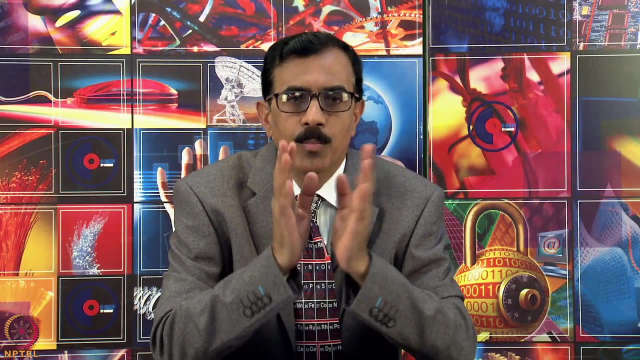 an encapsulated noble gas gas atom in a void in the lattice was I have shown here. So hydrogen atoms of water molecules are omitted for clarity. just I have shown here oxygen and you can see here this group, 18 element xenon sitting here in the void. So noble gas halides are quite well known. they are important class. 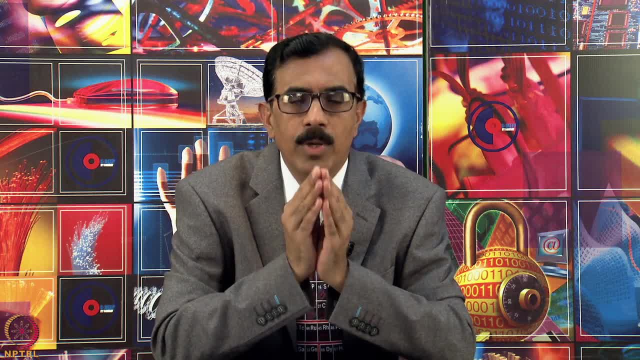 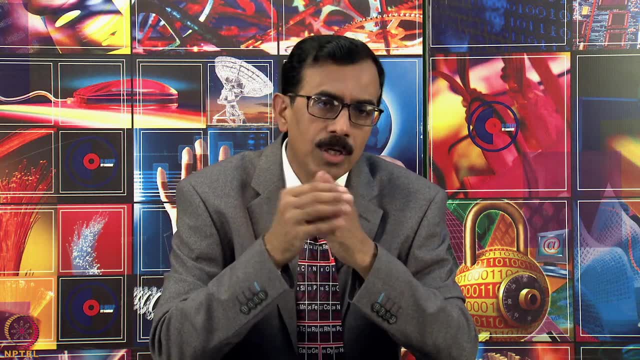 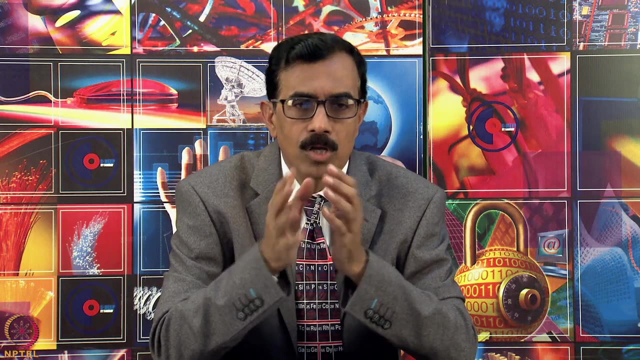 of compounds. Fluorine is the most electronegative element and is able to stabilize the highly oxidizing noble gas compounds. most of them are essentially fluorides. The vast majority of compounds are fluorides of xenon. a few of krypton are also known, as I said, Though some chemistry of 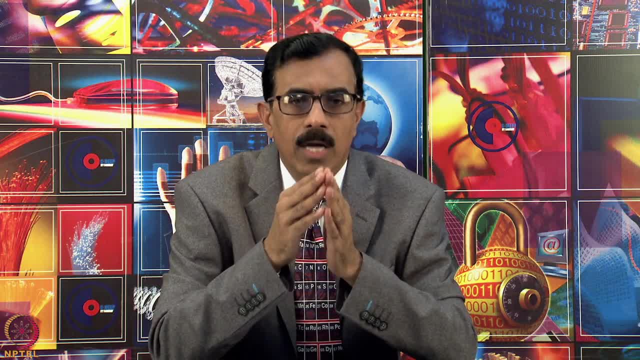 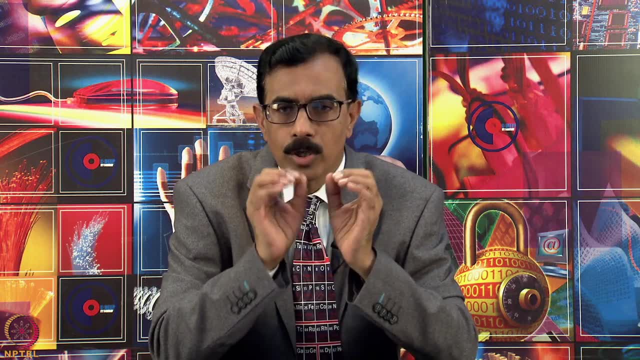 radon is known, hampered by its radioactivity and availability in very small or trace amounts. So noble gases are used as low temperature refrigerants to provide an inert atmosphere, and liquid xenon is used to provide an inert atmosphere and liquid xenon is used to provide. 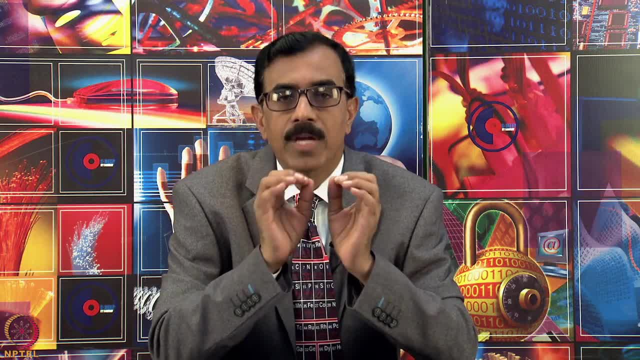 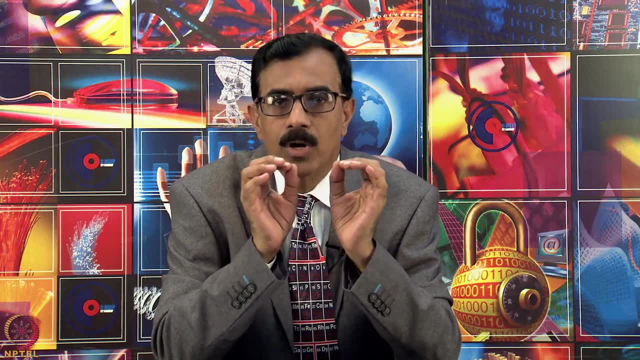 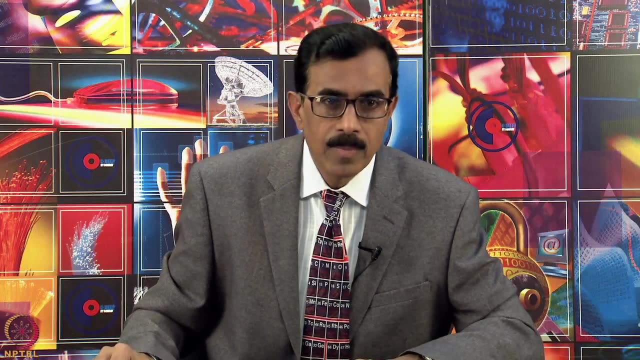 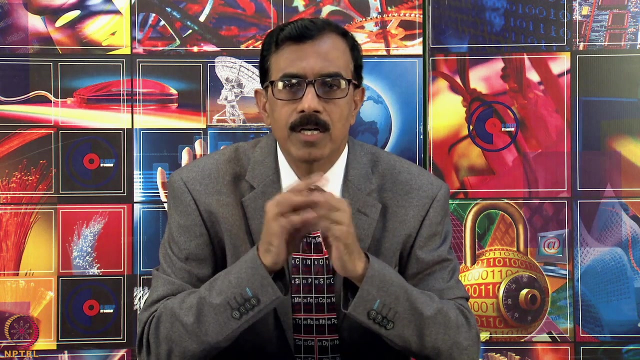 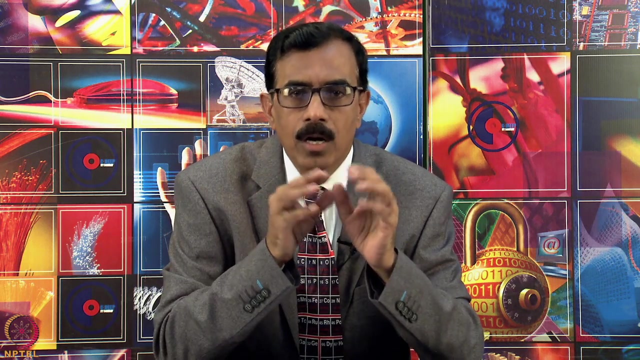 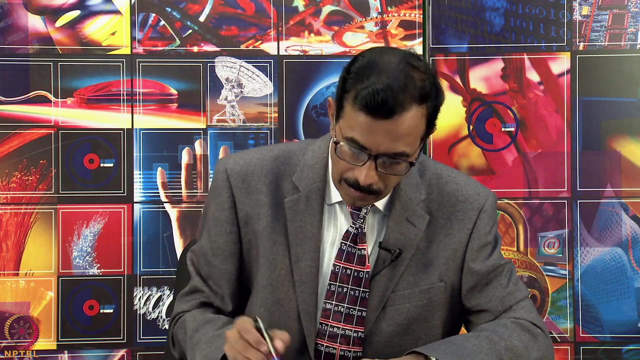 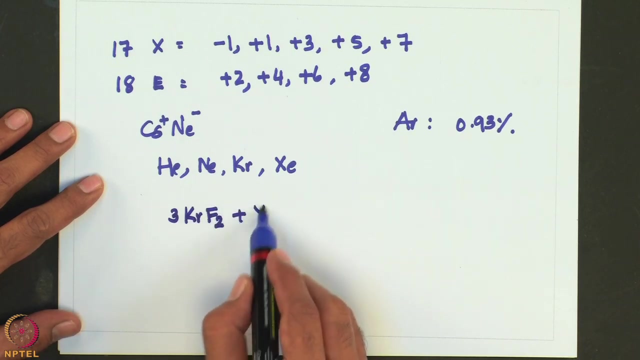 a beastly radiantітat to xenon hexafluoride and also metallic gold to gold hexafluoride anion. For example, 3 krf2 plus xc gives xcf6 plus krypton. 7 krf2 plus 2 Au gives 2 krf2 plus. 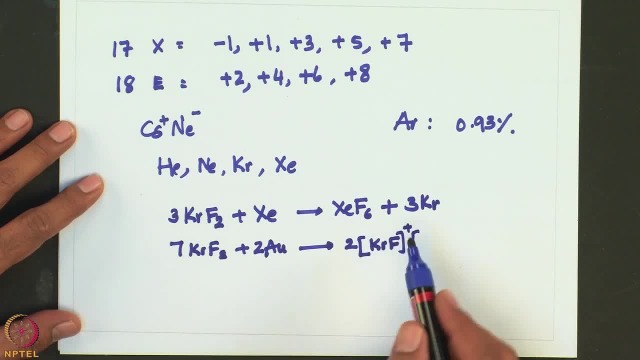 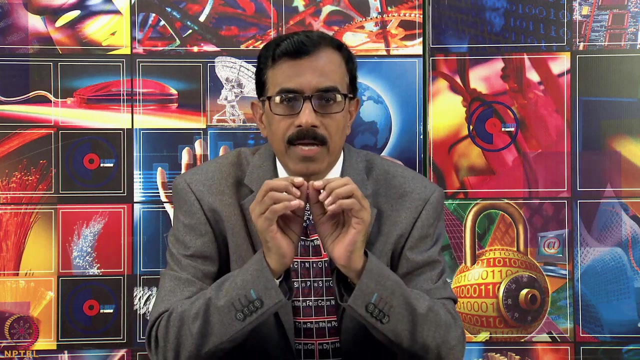 krypton is in plus 2 oxidation state: Au f6 minus plus 5 krypton. You can see here gold is in plus 5 oxidation state. Now let us look into xenon fluorides. A xenon fluoride xcptf6 was the first noble gas compound to be synthesized. 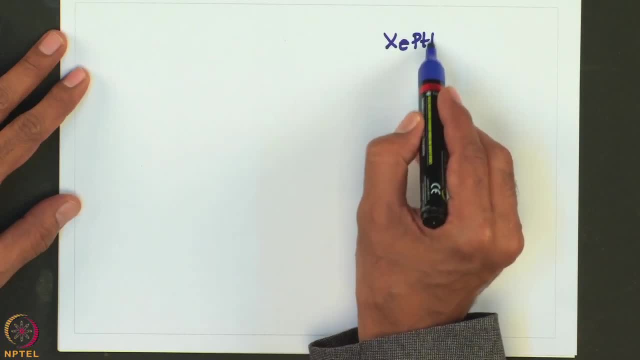 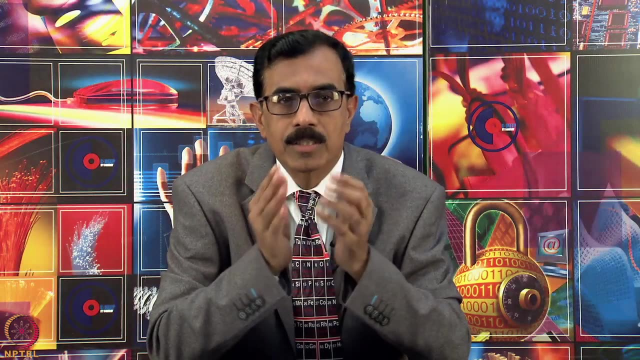 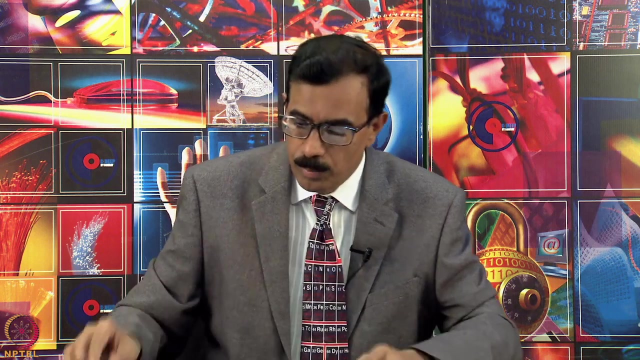 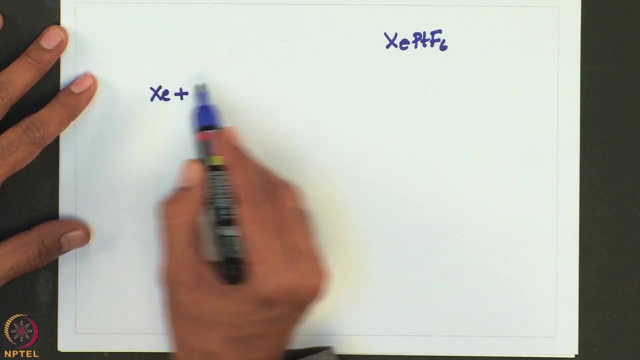 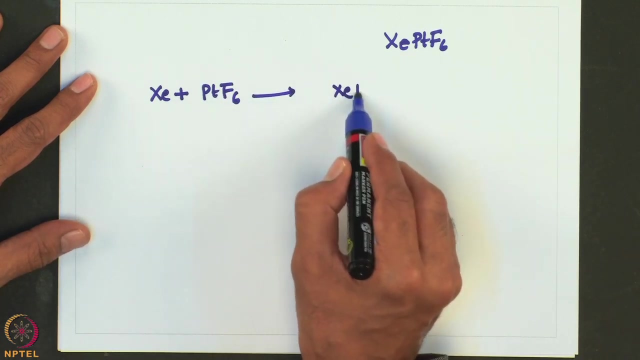 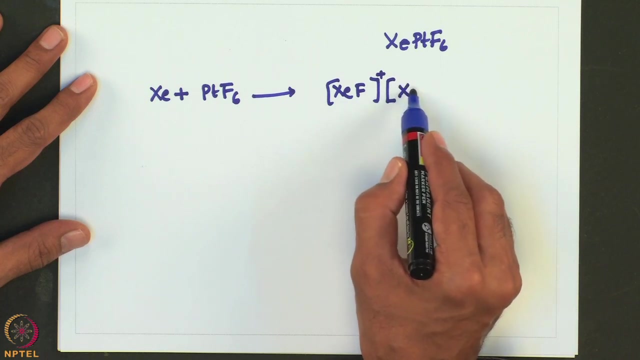 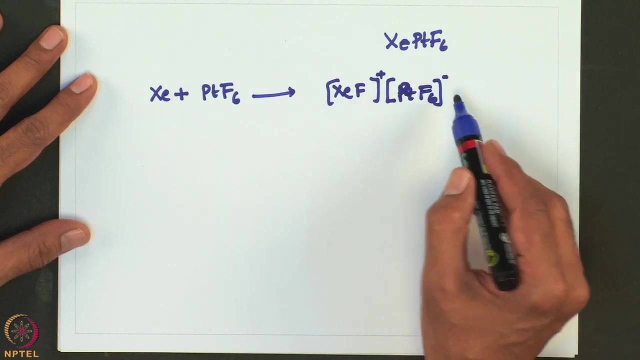 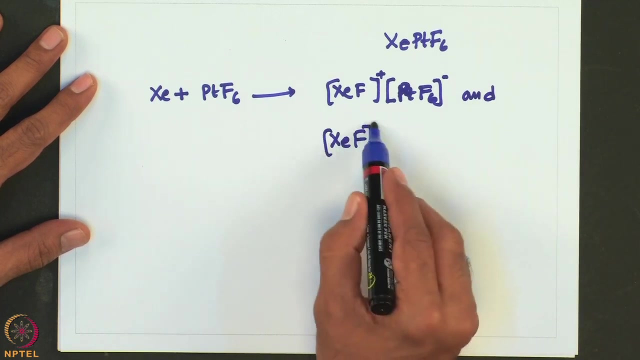 Ok, by reaction of xenon with strong oxidant such as ptf6, and it was later shown to be probably a mixture of xcf plus and ptf6 minus. So that is xenon plus ptf6 which was shown. So you can see that it was as common as xcf plus and ptf6 minus, and also xcf plus and pt2f11. 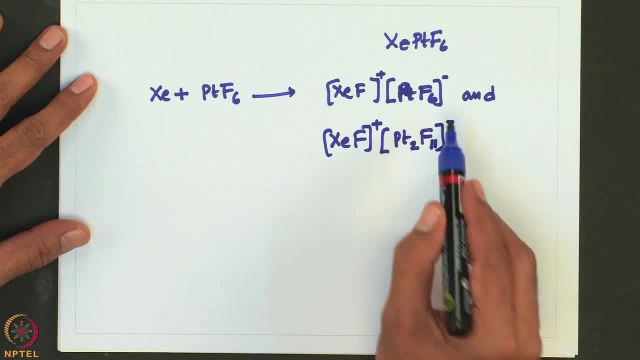 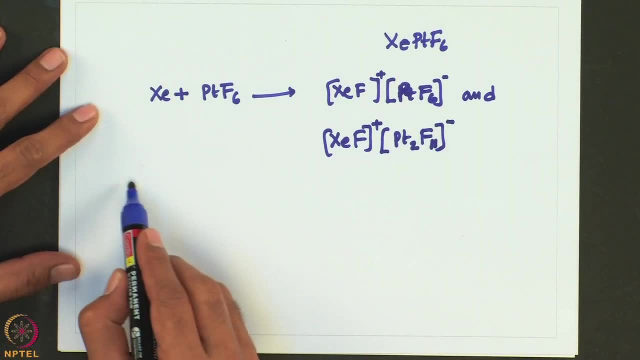 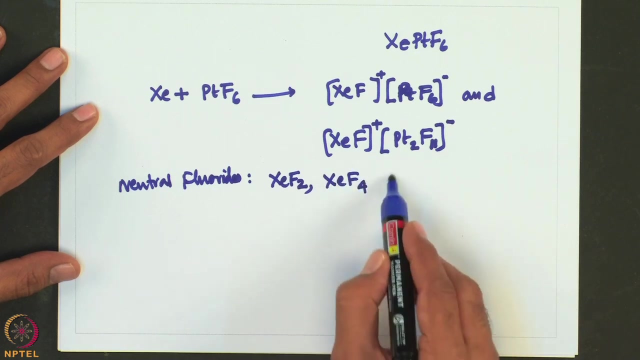 minus. Ok, So just Ok, Thank you very much. Okay, Ok, So xenon forms 3: neutral fluorides, xenon difluoride, xenon tetrafluoride and xenon hexafluoride. ok. 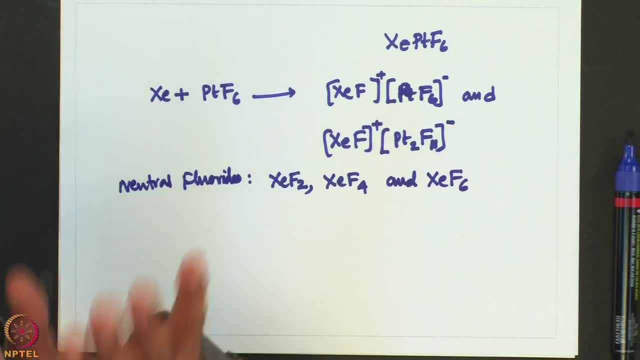 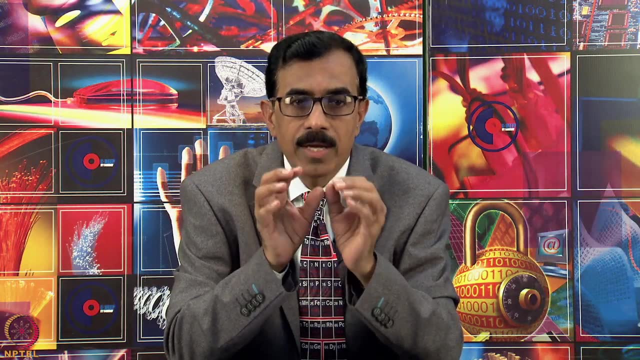 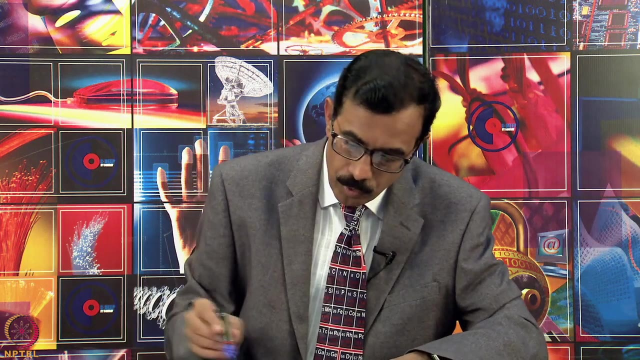 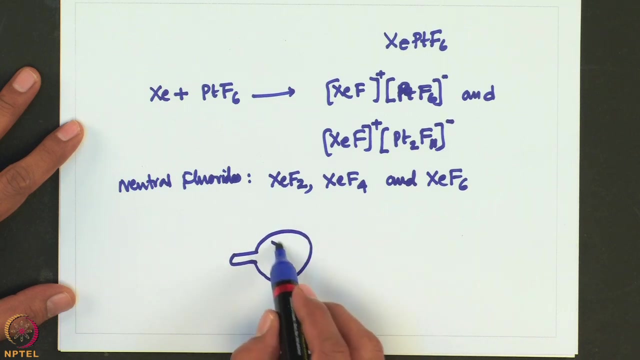 By the reaction of fluorine and xenon under different reaction conditions. simplest method involves exposing a fluorine- xenon mixture in a dry glass bulb to sunlight. colorless crystals of XEF2 are deposited at the walls of the flask. What you can do is you can take a tube like this sealed one containing xenon and F2,. 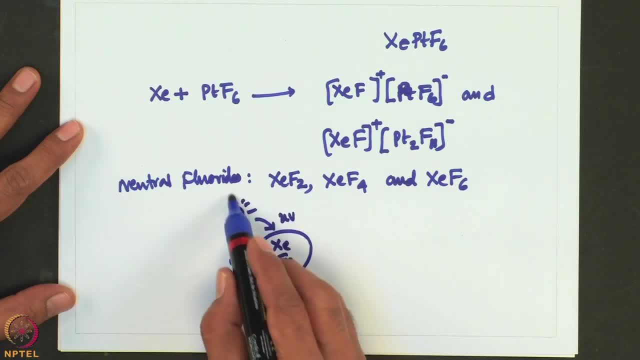 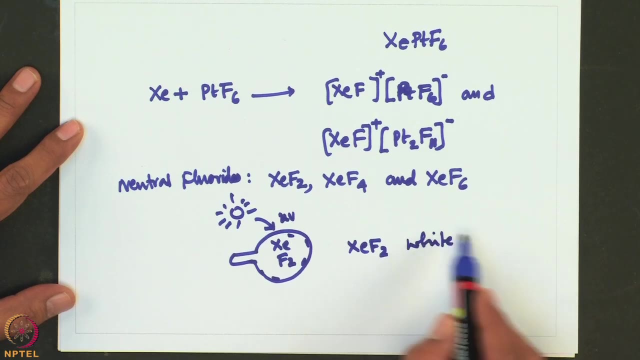 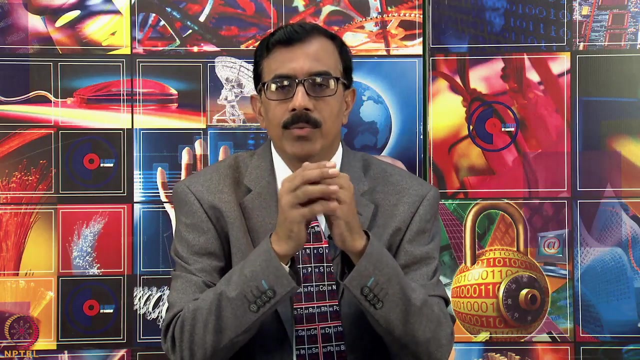 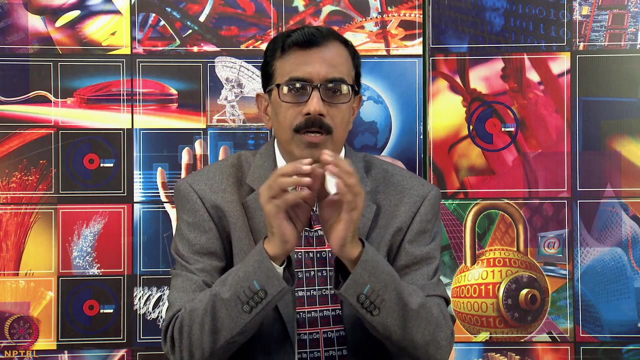 shine UV light, That is from sun. so it gives XEF2 in the sides here as white crystals. ok, The sunlight causes dissociation of the relatively weaker FF bond in F2 to form F atoms which then react with xenon. So with the ratios of fluorine to xenon higher temperature and higher pressure one. 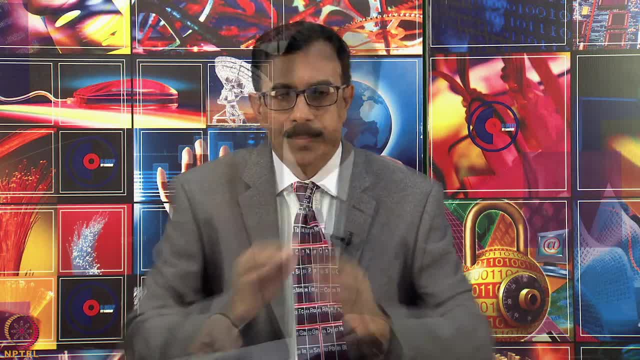 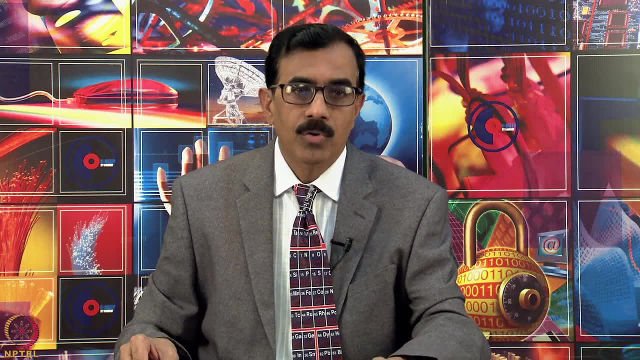 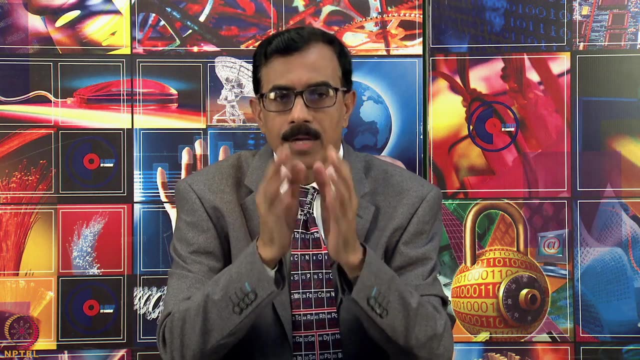 can make XEF4 as well as XEF6.. If you are curious to know the structure and geometries of xenon fluorides, of course you can always use VSEPR theory very effectively to arrive at the geometry and shapes of xenon. 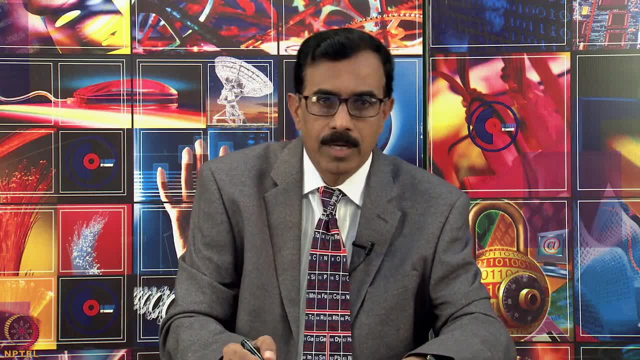 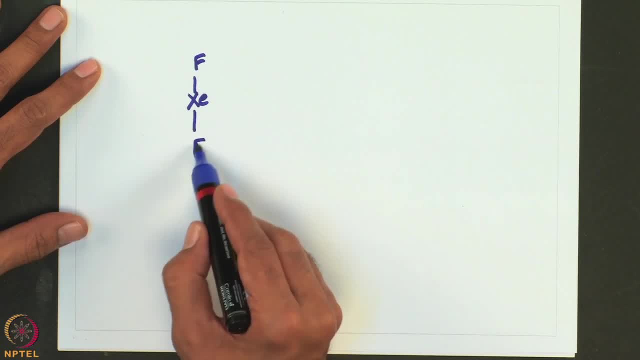 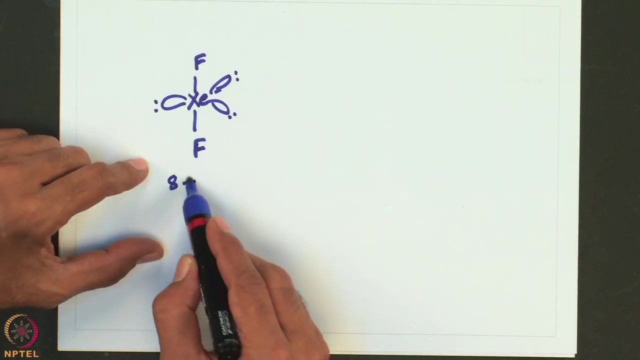 fluorides, For example, if you take xenon difluoride, It is linear, whereas the geometry is trigonal, bipyramidal. Basically, we have eight electrons are coming from this, one and one each. two electrons are coming. 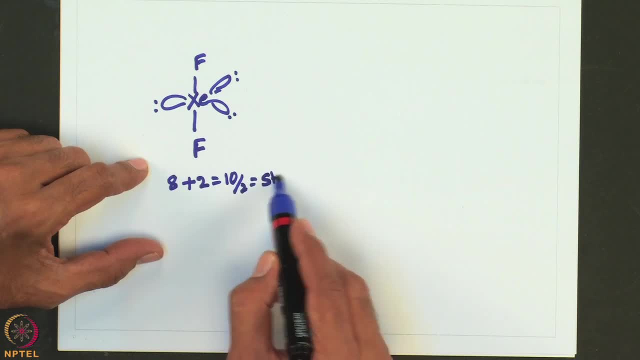 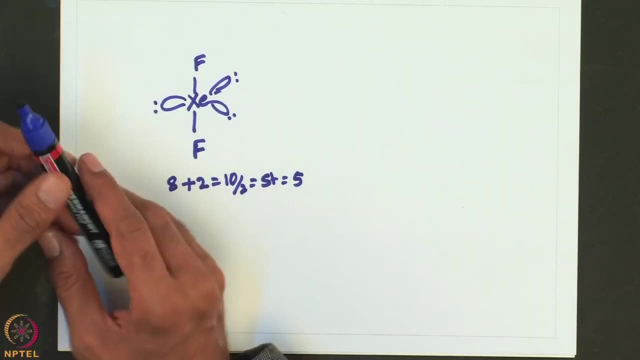 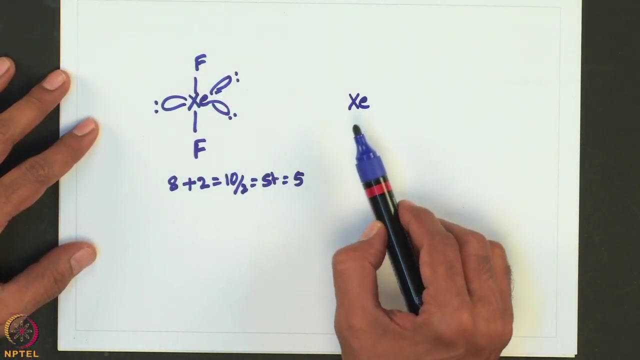 So we have ten electrons by two, Because steric number is equals 5.. 2 bonded pair and 3 lone pair. best geometry would be trigonal bipyramidal, ok, So similarly one can write for X e of 4.. So X e of 4, if you take again 8 plus 4, 12 electrons are: 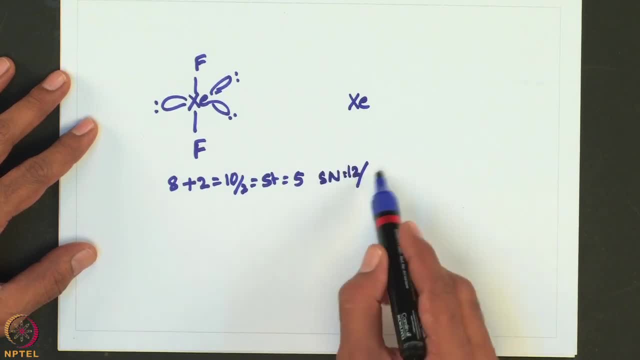 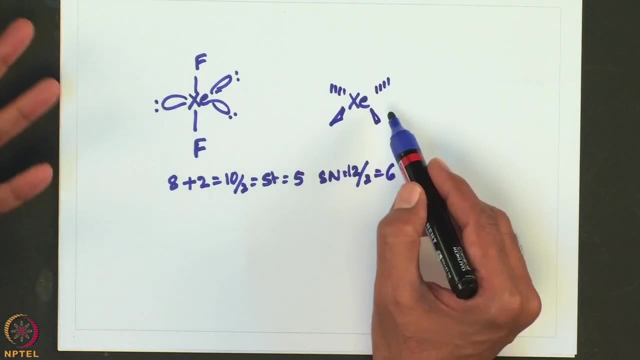 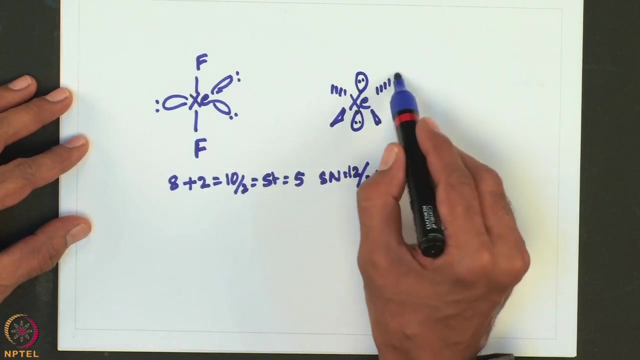 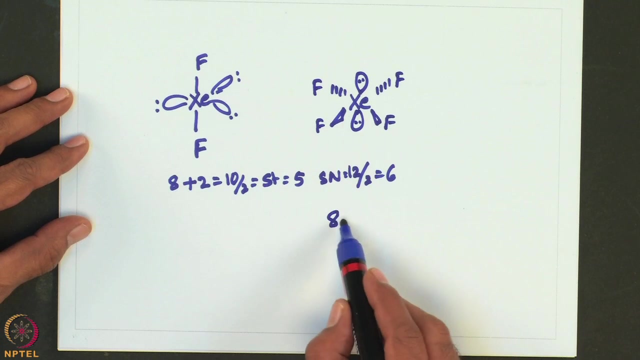 there. If 12 electrons is the steric number, that is 2 equals 6,. 4 bonded pairs are there and there have to be 2 lone pairs and structure has to be octahedral and the shape has to be planar. So here, 8 electrons are from xenon, plus 2 electrons are from 4 electrons. 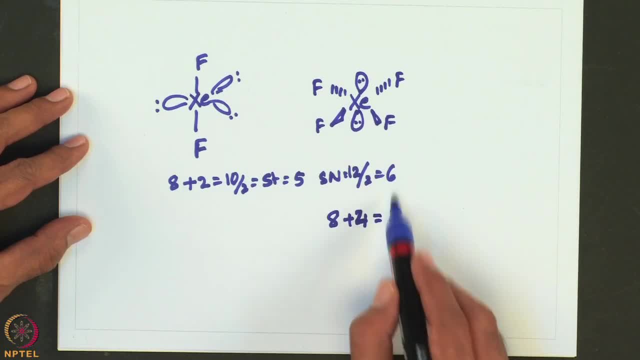 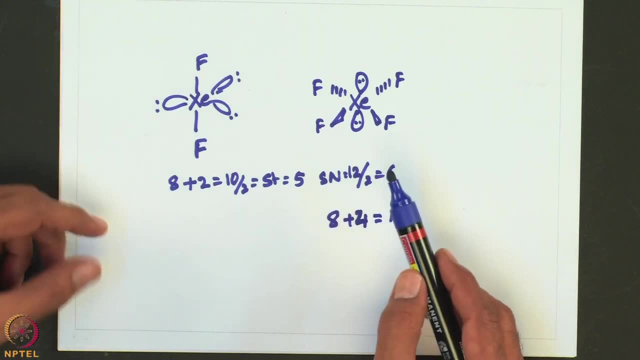 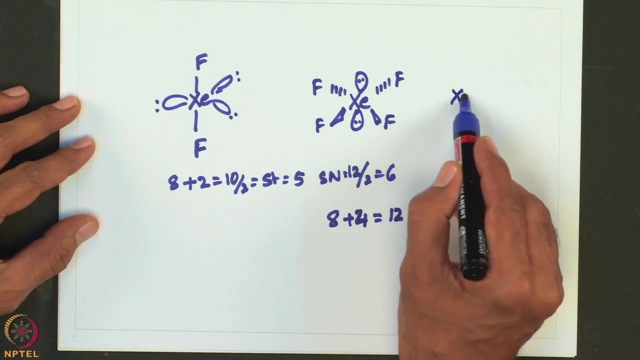 are from 4 fluorine atoms is 12.. So 12 is the total number of electrons. that steric number is 6.. So you have this octahedral geometry and planar shape. ok, Ok, When you consider X, e of 6.. So here, 8 plus 6 equals 14 electrons. are there, 14 by 2 equals. 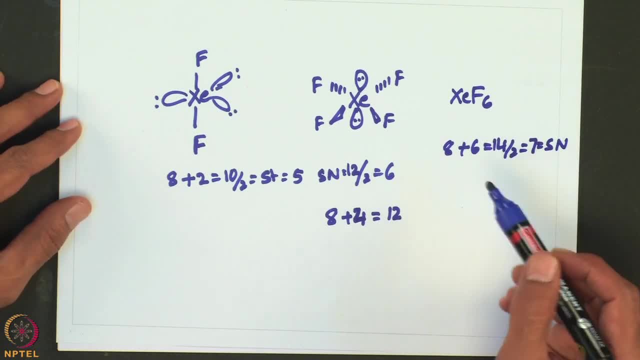 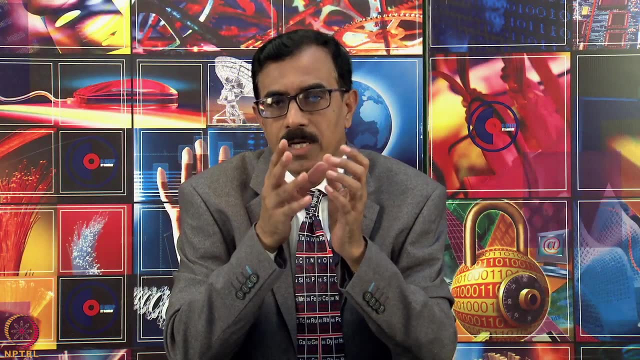 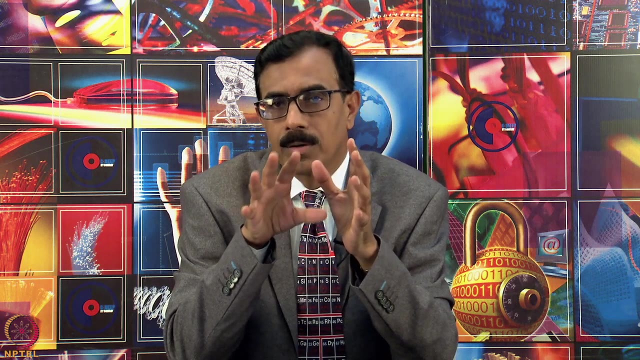 7 is the steric number. So here one lone pair is there. So this one lone pair occupies one of the triangular faces of octahedral. So that means essentially it becomes a capped octahedral geometry. but here it is delocalizing over entire octahedral geometry. So this: 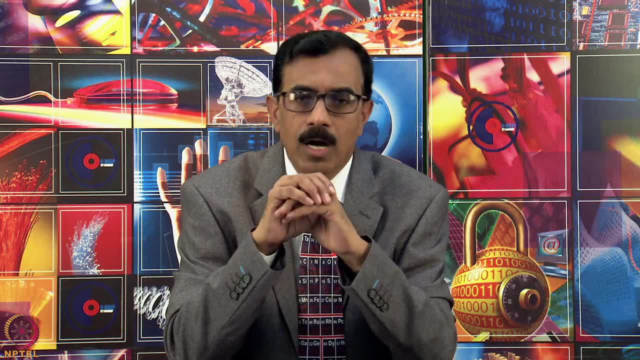 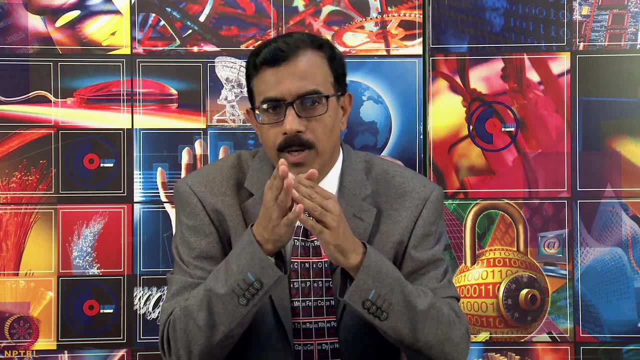 capped octahedral geometry. as a result it appears slightly distorted octahedral structure. So X e of 6 is fractional in the gas phase, So interchanging between the structures where the lone pair points through the centre of an F e triangle, as I mentioned. ok, So since 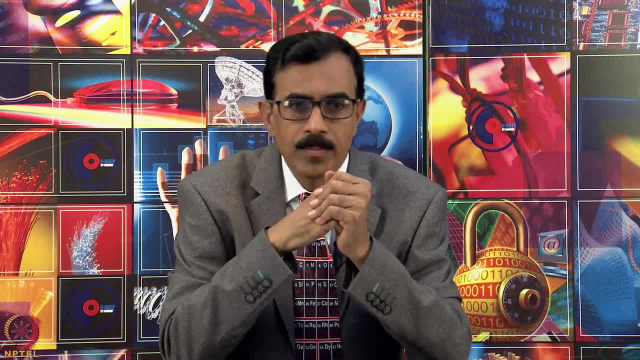 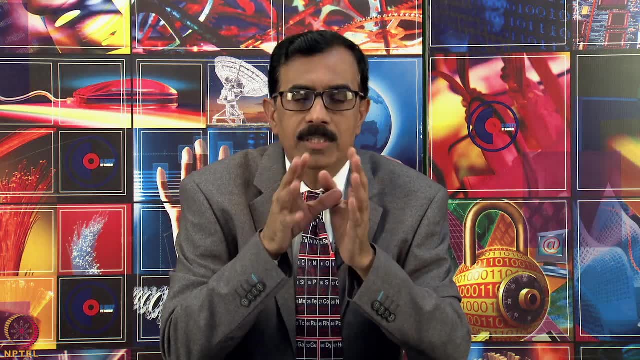 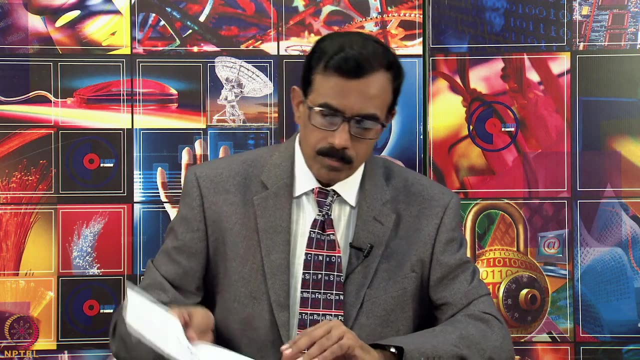 the lone pair is in a spherically inactive s orbital. what happens? it does not appear like typically a capped octahedral structure, but it appears like a slightly distorted octahedral structure. Ok, Of course I wrote. I am showing you here the structures. here you can see X, e of 2 and also 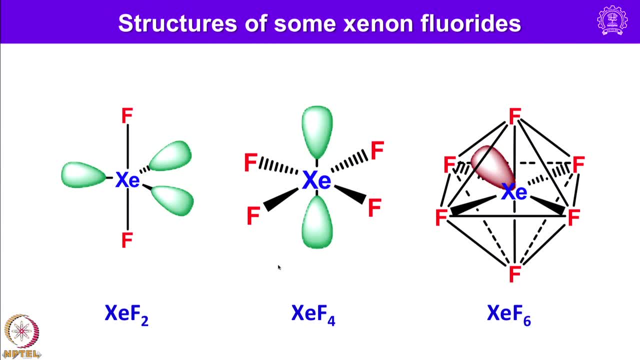 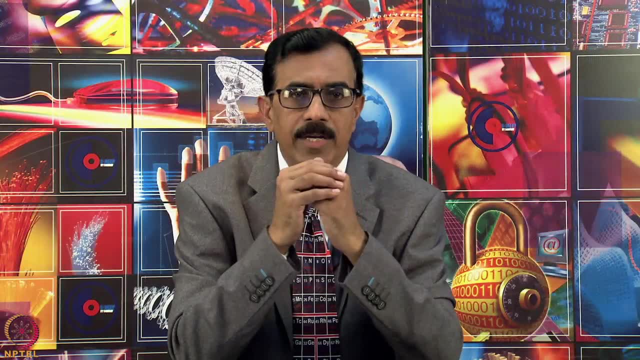 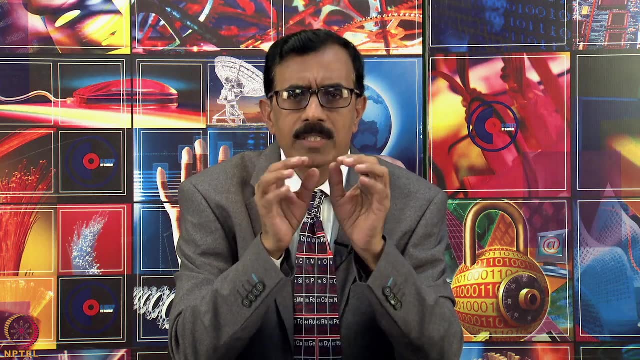 you can see X e of 4 and also you can see X e of 6 here. ok, This lone pair is represented here in this lobe here. So all of the xenon fluorides are powerful fluorinating agents able to oxidize a wide range of compounds. In many cases, X e of 2 is a very selective. oxidant, So it can oxidize the central hetero atom of a main group compound like arsenic, phosphorus and etcetera, but not the organic substituents bonded to it. For example, if methyl or phenyl groups are there, they are not getting fluorinated. only the central atom is getting fluorinated. 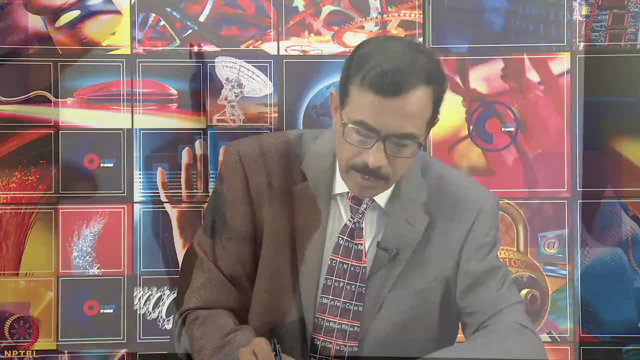 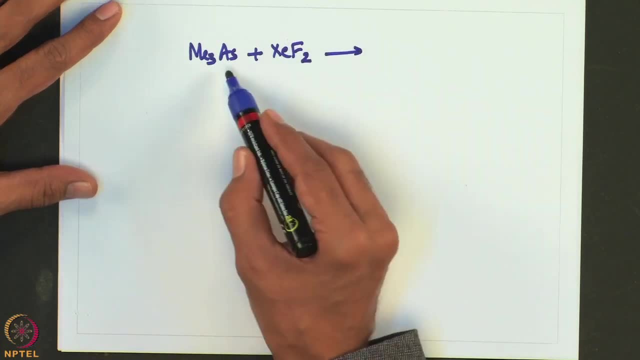 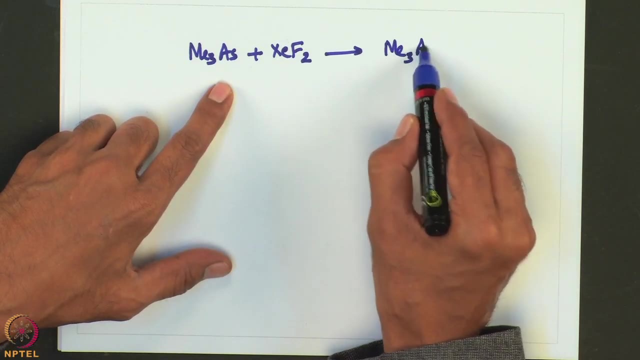 Let me write couple of examples. For example, if I take trimethyl arsine and treat with X e, F 2, only here arsine is getting fluorinated. So it is getting fluorinated to form pentavalent, pentacoordinated trimethyl difluoroarsine. 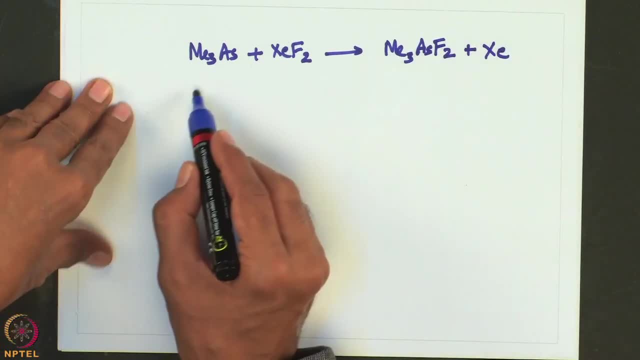 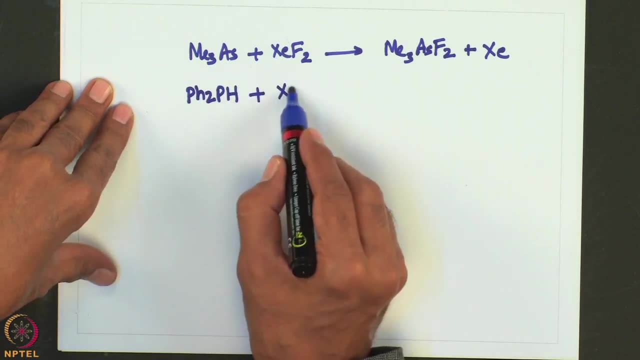 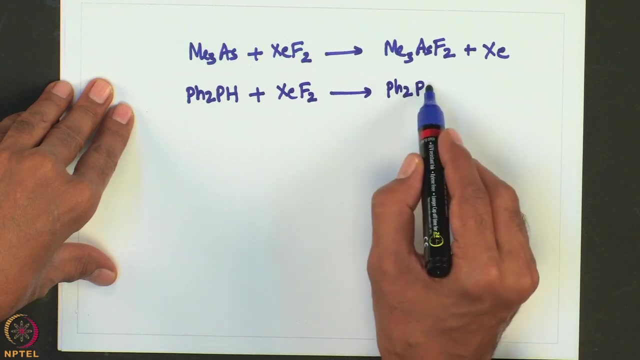 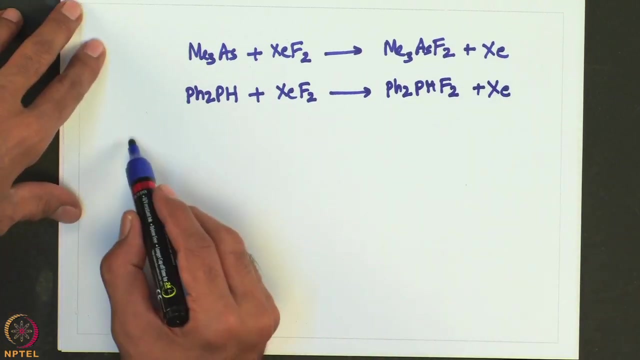 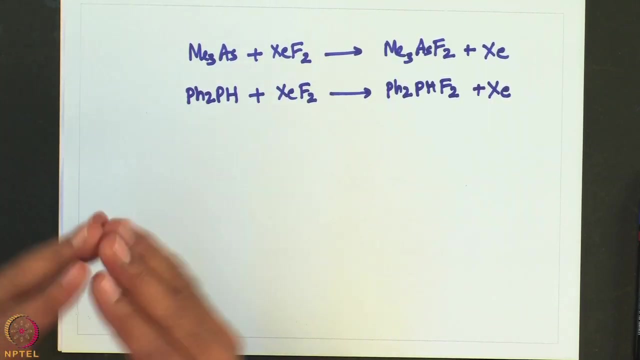 Similarly, if diphenylphosphine is treated with xenon difluoride, again here phosphorus getting fluorinated, So we get pH 2, p, H, F, 2. Plus xenon. So X e F 2 also oxidizes water to oxygen, while X e F 4 can oxidize platinum. 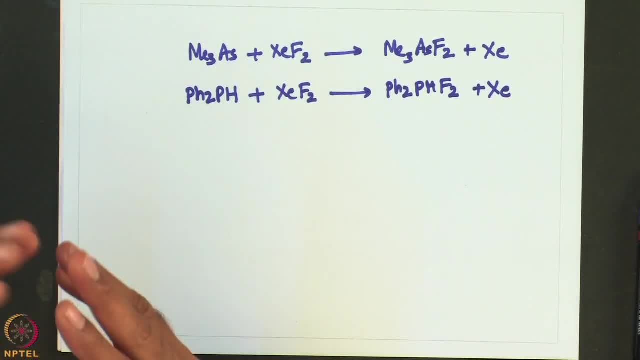 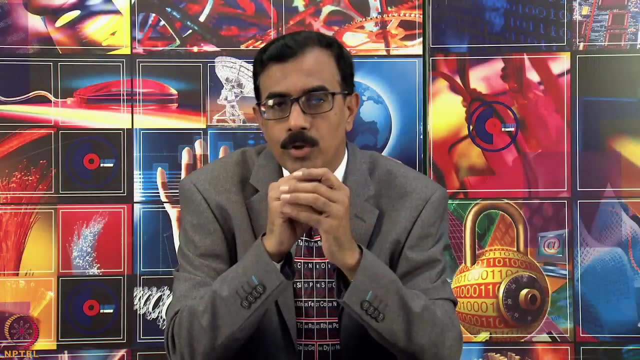 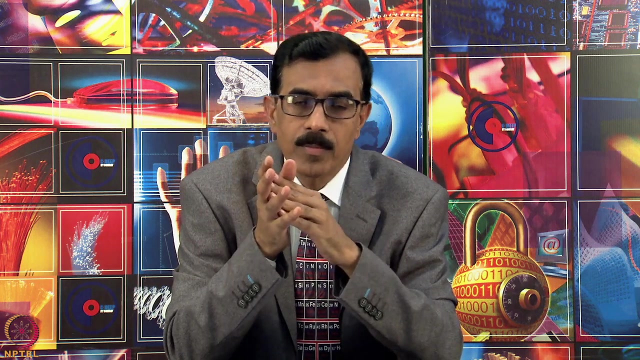 metal to P, T, F, 4.. So why we say oxidation of oxygen in water? Because if you just look into water, oxygen is in 2 minus state and in when it is decomposed and we get oxygen, oxygen is in 0 valence state. So it is in 0 valence state. So it is in 0 valence state. 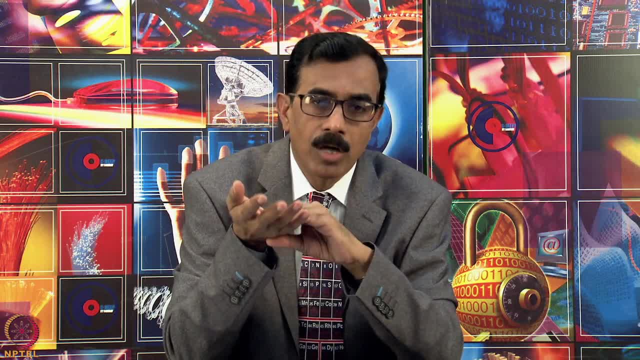 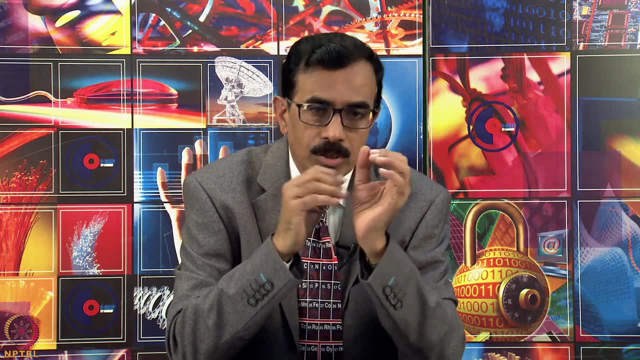 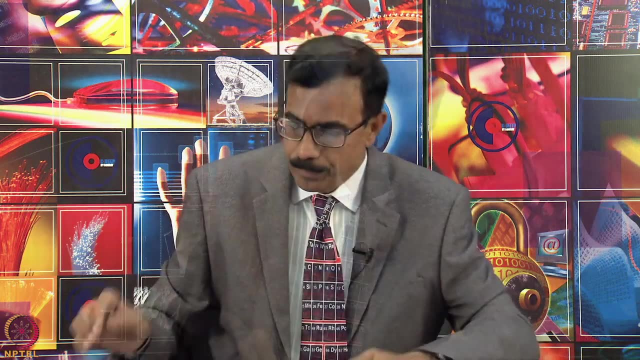 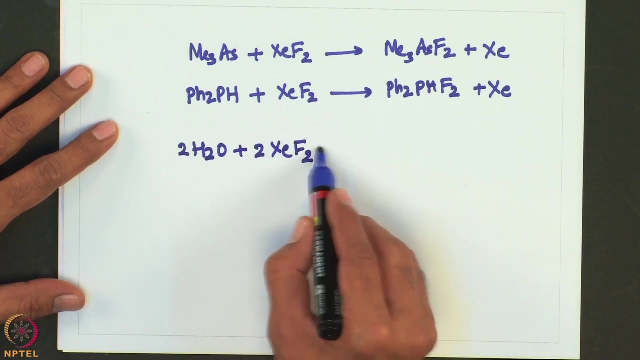 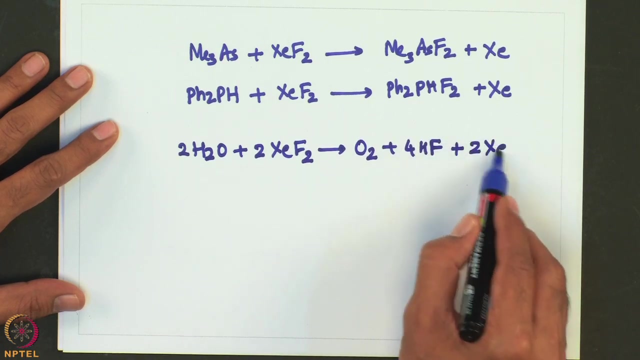 Essentially it is oxidation of oxygen if water is dissociated or broken up. So here, xenon difluoride oxidizes water to oxygen, while X e F 4 can oxidize even platinum metal to platinum tetra fluoride. Similarly, if you take X e F 4 and treat this one with platinum metal, It gives platinum. P, T, F, 4 with platinum is in plus 4 state plus xenon. Novel gas fluorides can react with fluoride ion donors as well as acceptors, and the chemistry is quite extensive. So noble gas fluorides react with strong fluoride ion acceptors, such 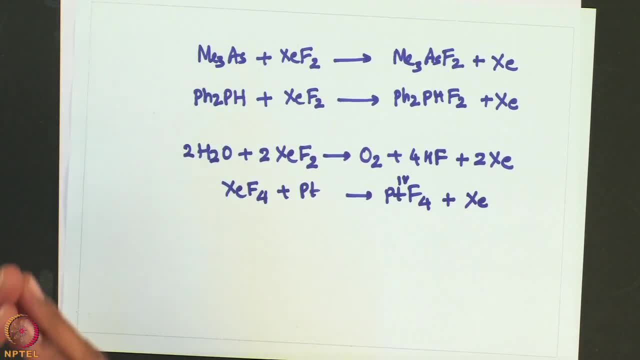 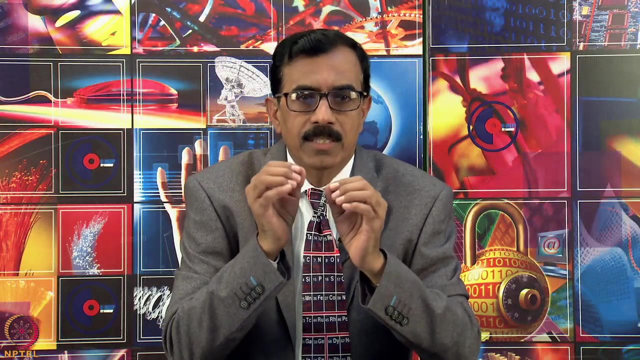 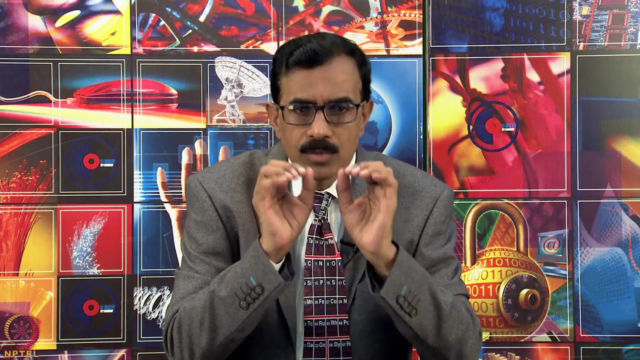 as group 15, pentafluoro derivatives of arsenic, antimony, bismuth, and also tantalum, ruthenium and platinum. Xenon difluoride forms the greatest number of compounds by this type of reaction, followed by XEF6 and XEF4 and KRF2. krypton difluoride forms many similar compounds, While 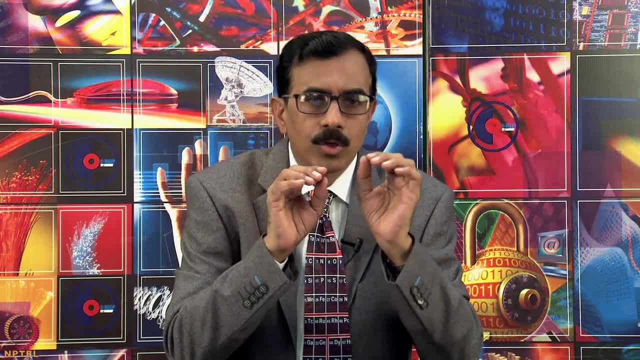 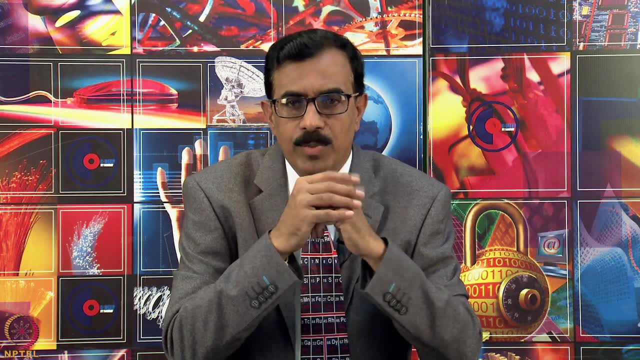 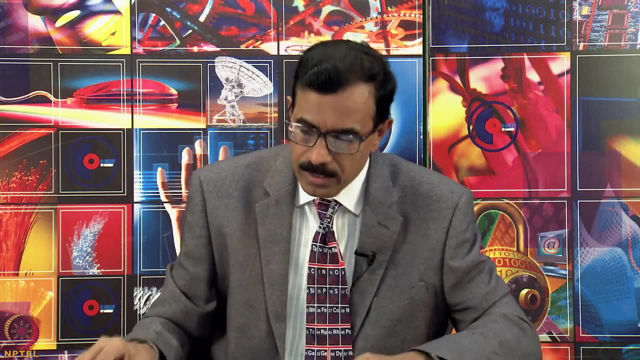 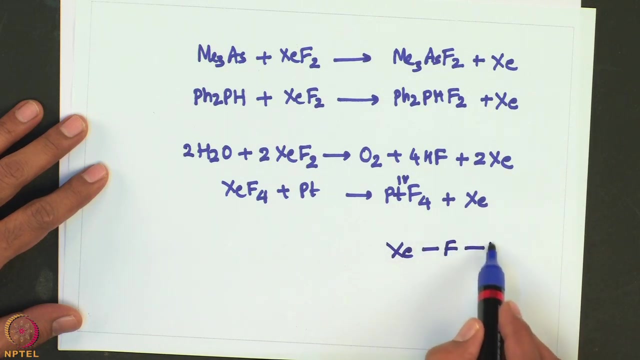 transferring the fluorides can be fully transferred to the Lewis acid, that is, MF5,, for example ASF5, SBF5, leaving cation xenon species. but in most cases fluoride is only partially transferred, resulting in compounds having XEF bridges, So fluoride bridges. So here 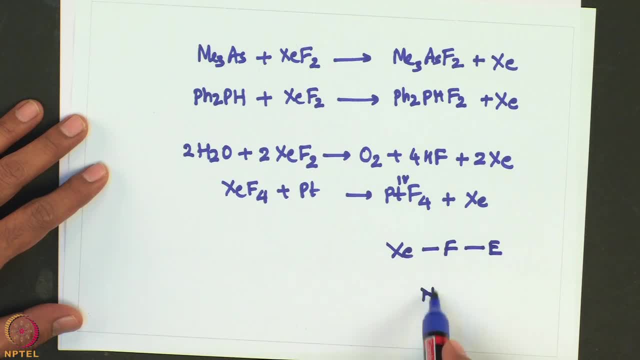 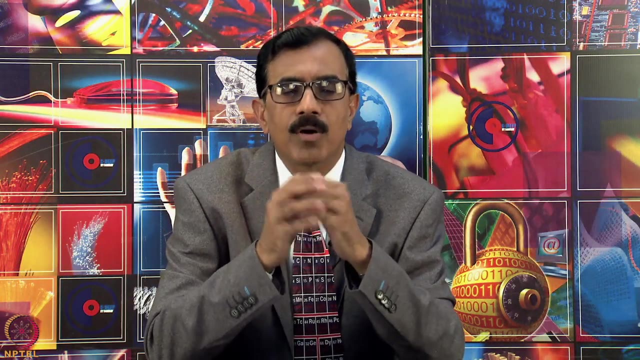 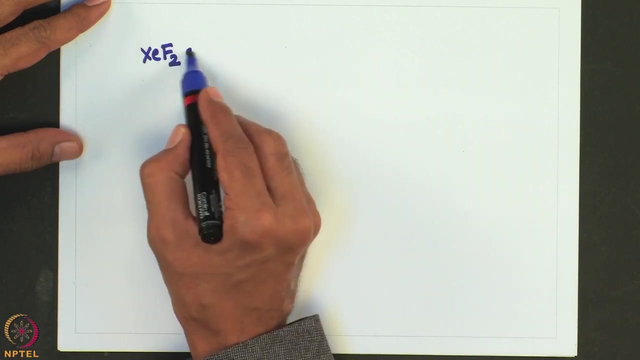 we have a fluoride bridge, So that means essentially Something like this in all these compounds where there is a partial transfer of fluoride. So different types of cations and anions are formed depending on the stoichiometry of noble gas fluoride. For example, XEF2 taken solid and treat this one with again fluoride. 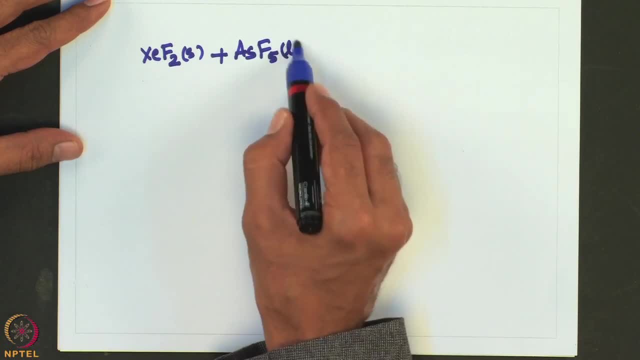 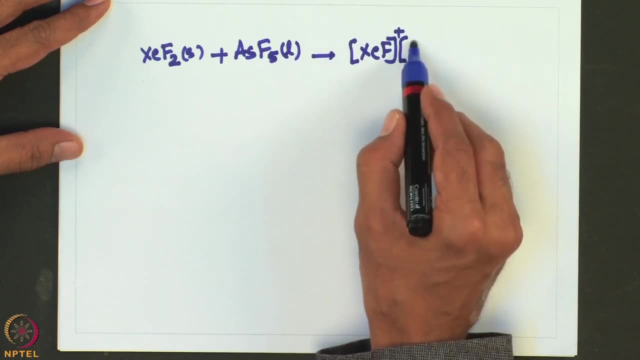 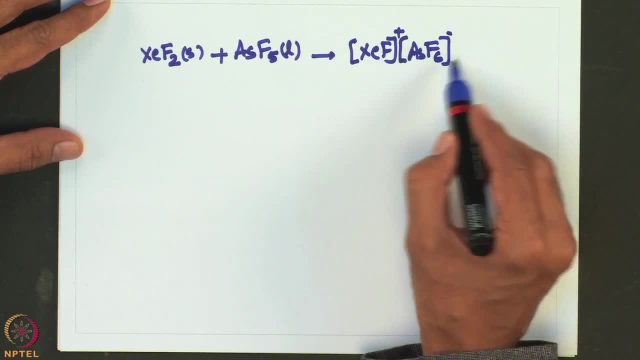 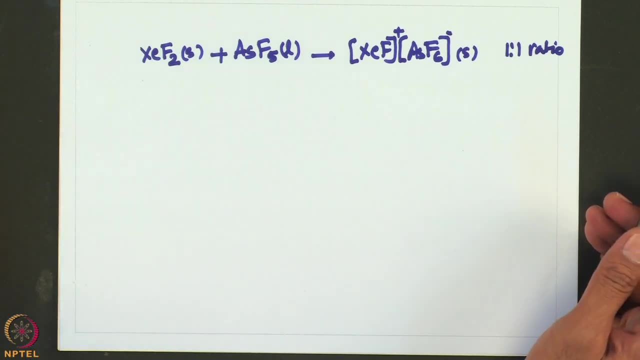 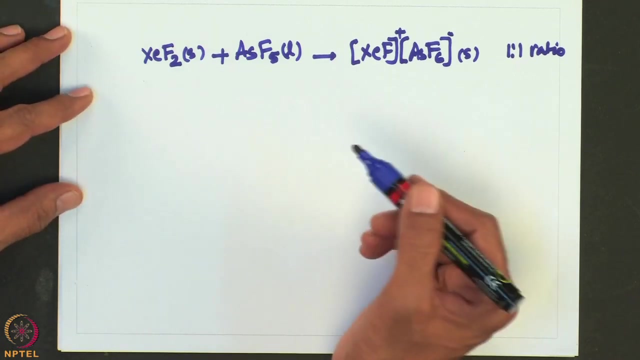 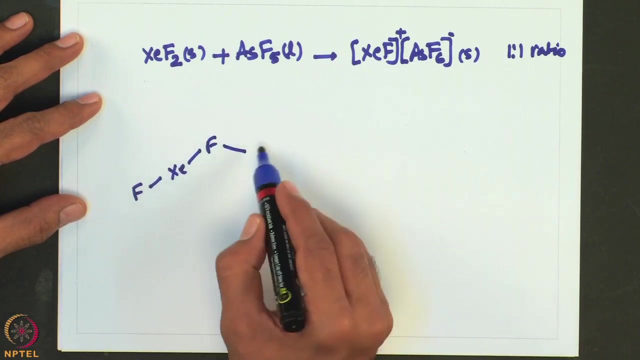 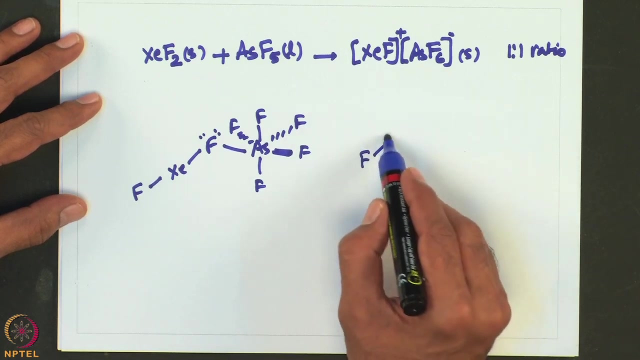 So what would happen when one is to two ratio is used, So we can have more of them, For example? I will write some of the structures here. Yes, Yes, You can see here partial transferring is there. This is X, c of A, s, f, 6 and also. 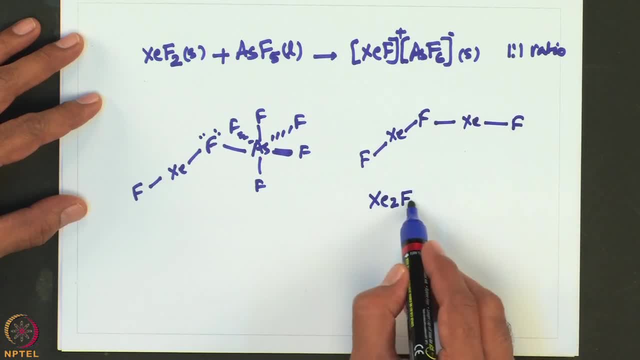 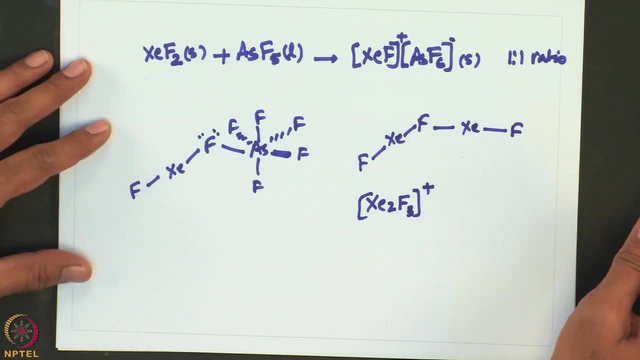 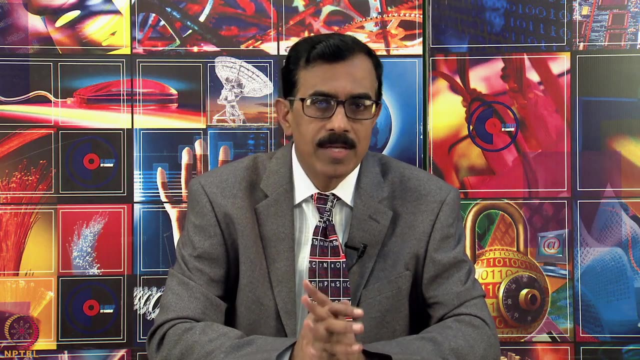 so we can also have X, c, 2, F, 3 cation and similarly we can also have a dimeric species, S, b, 2, F, 11 anion. Noble gas fluorides can act as fluoride acceptors or donors to give anions or cations. 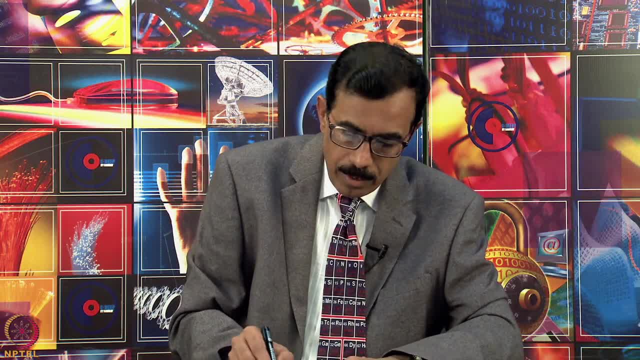 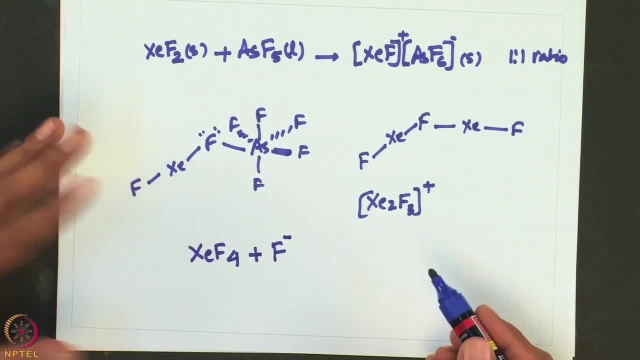 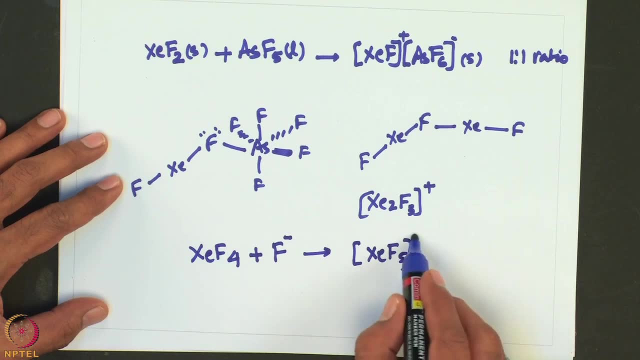 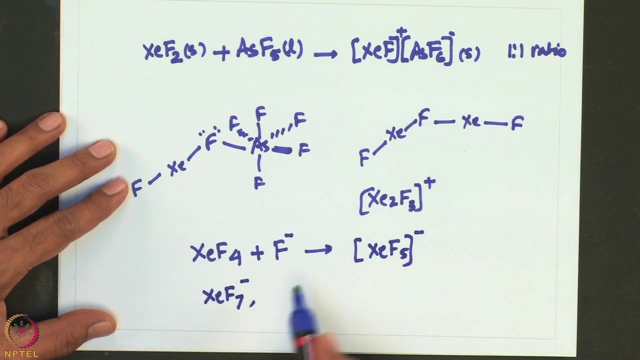 I already mentioned. Let me show you a couple of reactions here. For example, X c of 4. when it is treated with fluoride ion donors, such as cesium fluoride, it forms xenon pentafluoride anion. Similarly, X c F 7 minus. X c F 8 minus are known. they: 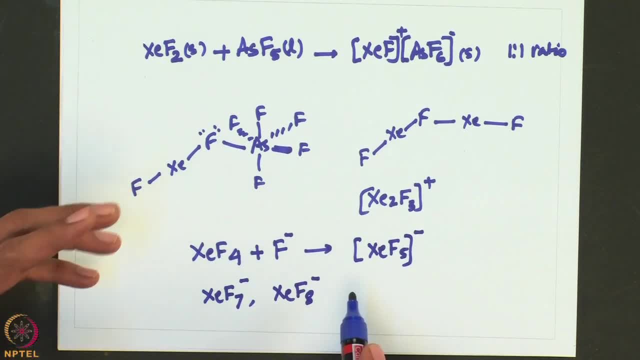 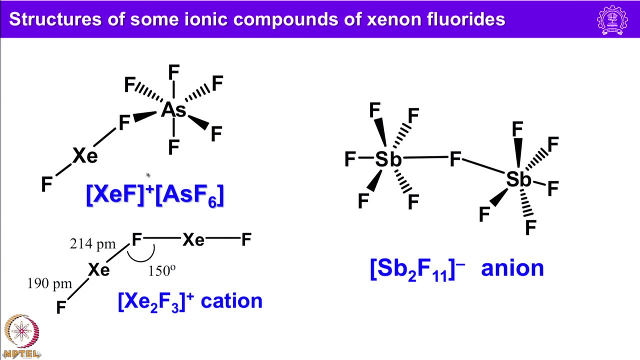 are obtained from X c- F 6 and X c- F 7 by adding 1 or 2 fluoride ions, The structures I have shown here for X c- F 7.. The F A, s, f 6 and also X c 2, F, 3 plus, and here this for S b, 2, F, 11 anion, So always. 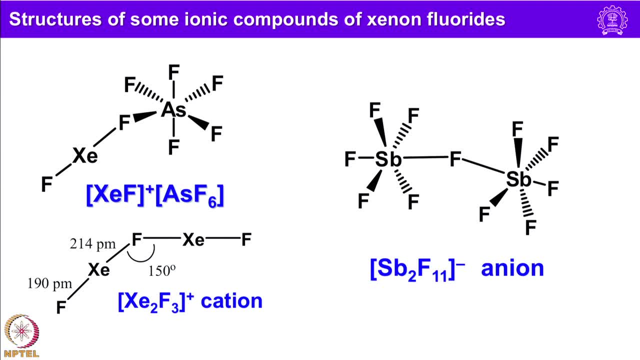 whenever these halides are bridging, you should never write in the stride and it should be at an angle. that angle will be much closer to the tetrahedral angle, because each bridging die, bridging halide ion, has two lone pairs intact on it. 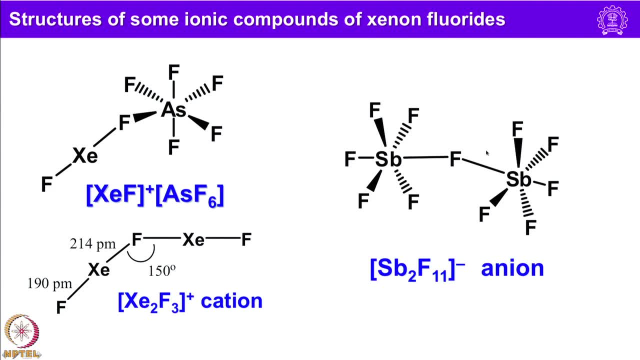 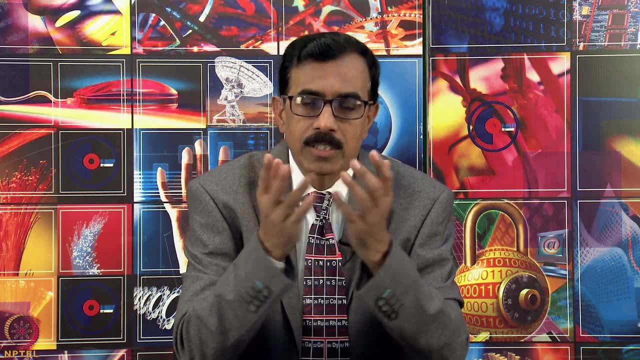 For example, in this case You have one lone pair here and one lone pair here. So xenon oxygen compounds are also quite known. They result from the hydrolysis of the fluorides such as X c F 4 and X c F. 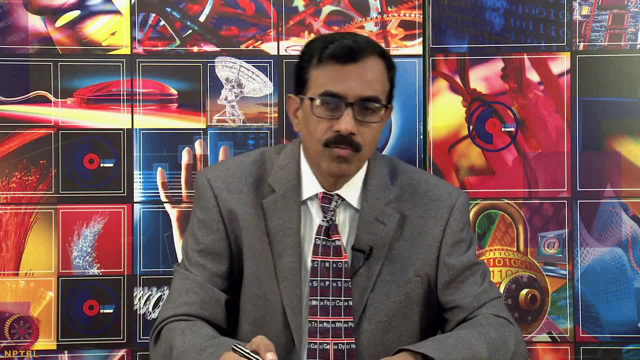 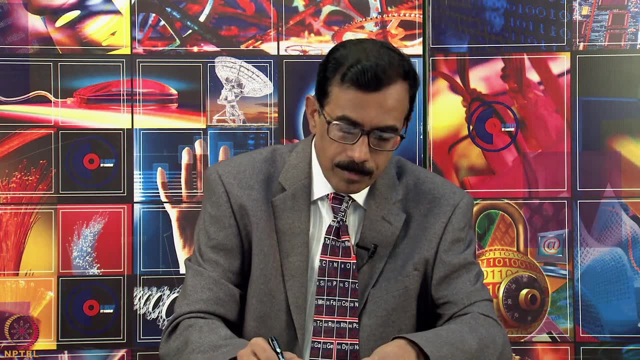 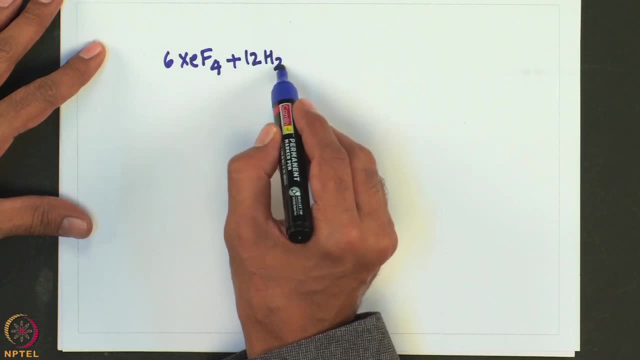 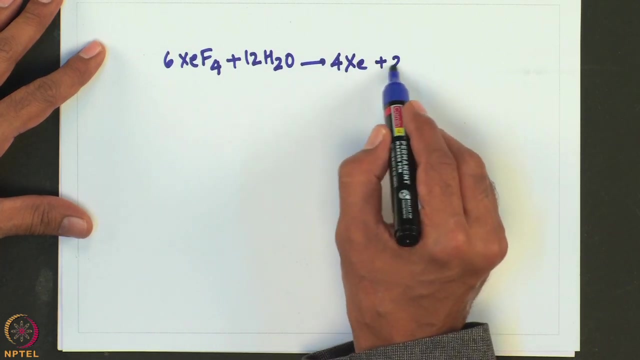 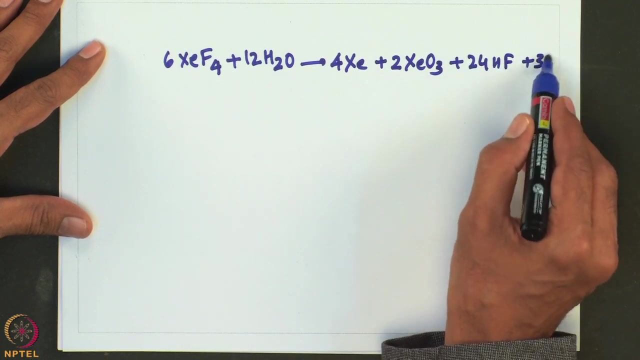 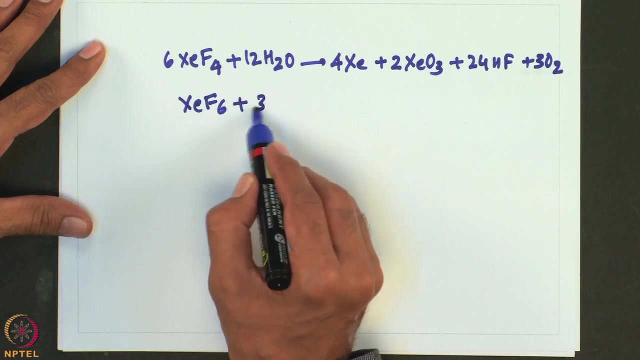 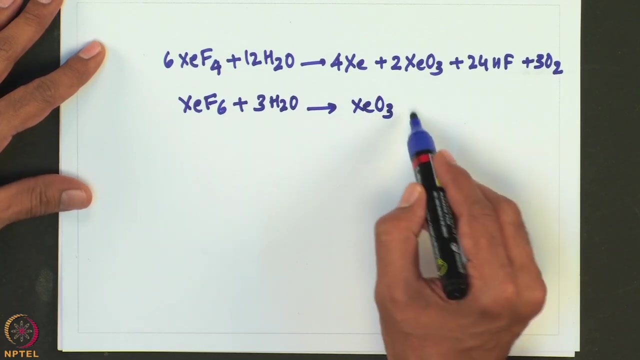 6.. For example, let us take xenon tetrahedral fluoride and try to add water to hydrolyze it. ok. Similarly, if you take X, c, F, 6 and treat this one with water, it undergoes hydrolysis to form xenon oxide plus 6 H F. 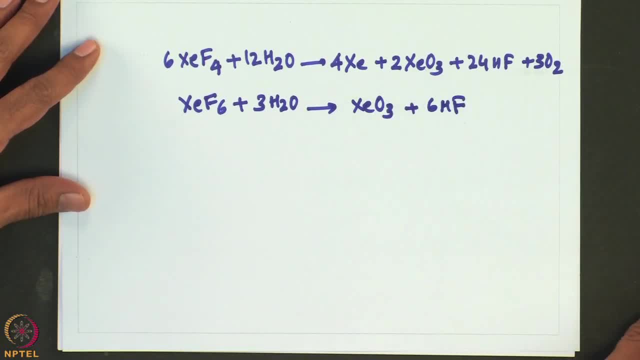 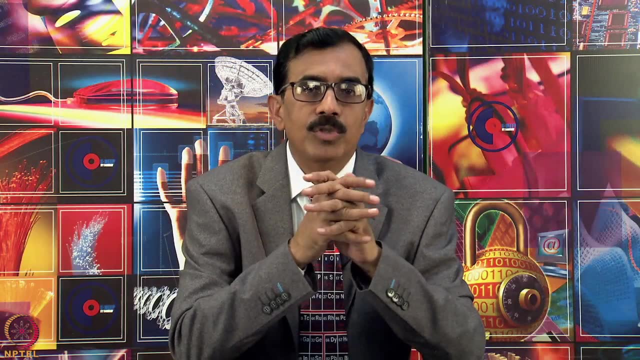 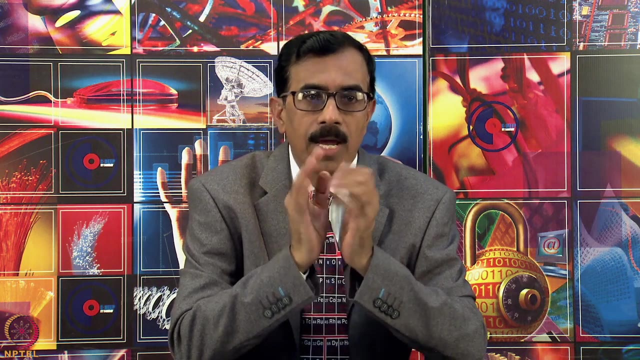 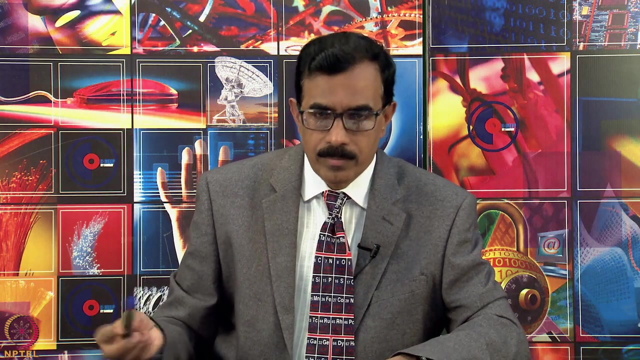 In this, in both, of course. here xenon is in plus 6 oxidation state. ok, So X c O 3 is a highly explosive white solid soluble in water. In strong alkaline solution X c O 3 behaves as a weak acid giving xenon 6 anion. So for 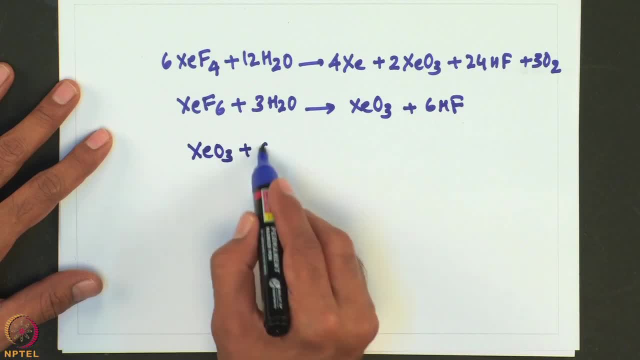 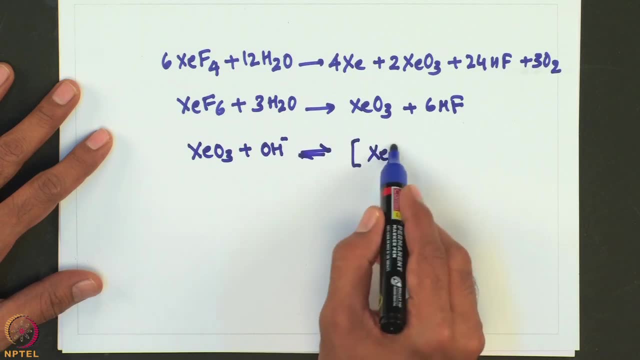 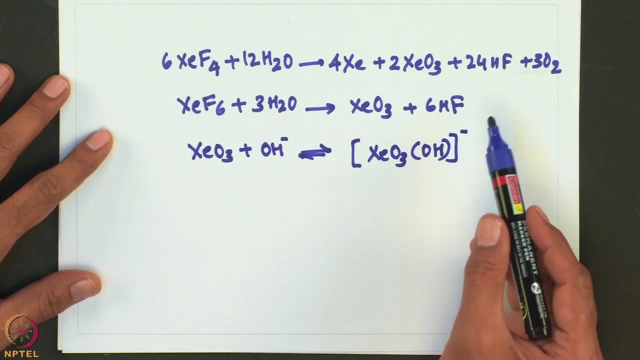 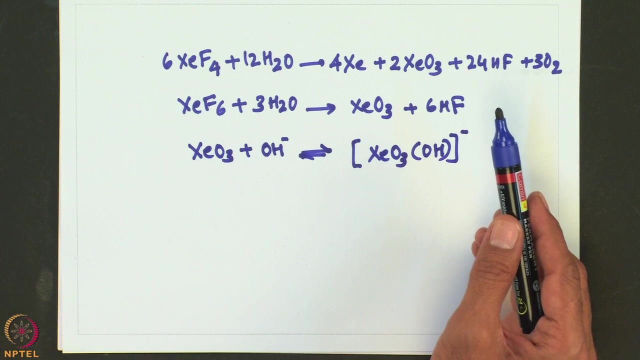 example X, c O 3. when it is treated with O H minus it gives xenate anion. So xenate anion is unstable in aqueous solution and undergoes a disproportionation reaction to give xenon gas and the xenate anion with xenon in plus. 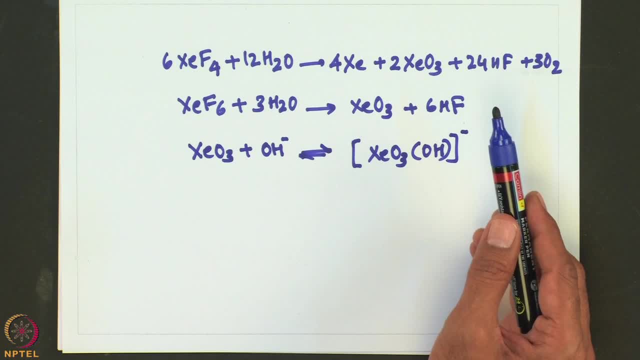 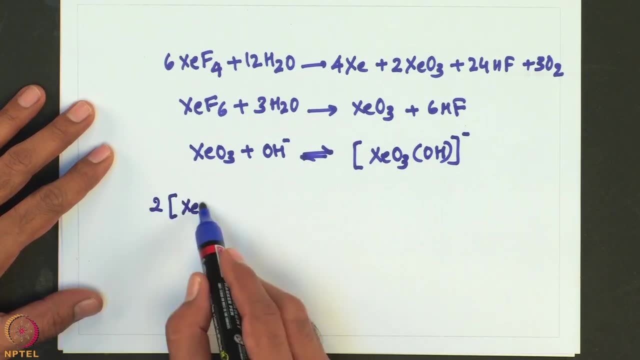 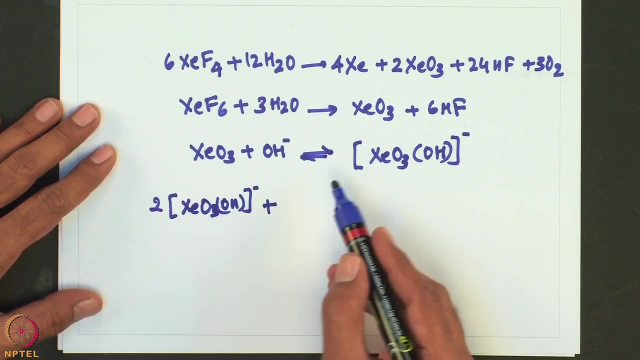 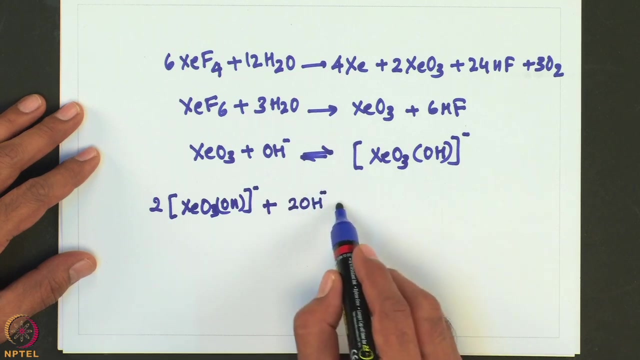 8 oxygen state, that is XeO6 4 minus, which contain xenon in plus 8 oxygen state. For example, if you take XeO3OH anion in aqueous solution, it forms XeO6 4 minus plus 8 oxygen. 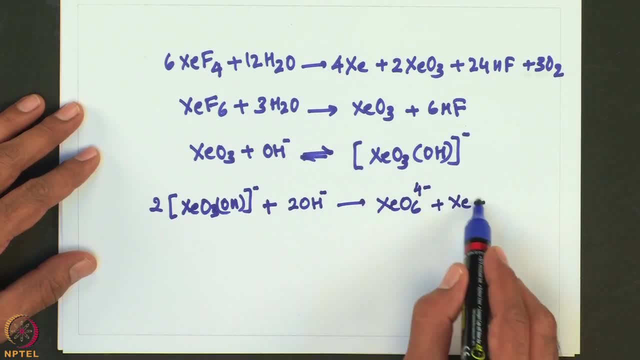 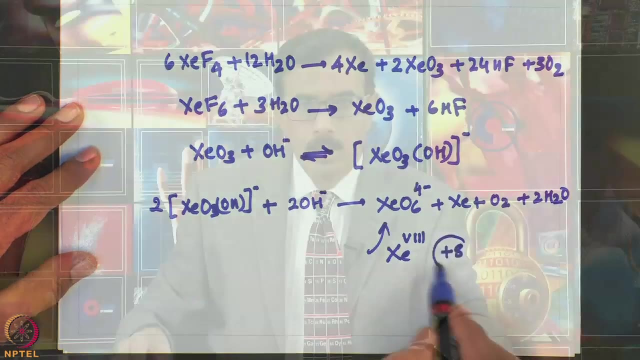 state plus xenon, plus O2, plus 2 H2O. So here xenon is in, is essentially xenon is in, plus 8 oxidation state. The controlled reaction of xenon hexafluoride with water will give xenon oxy fluoride. 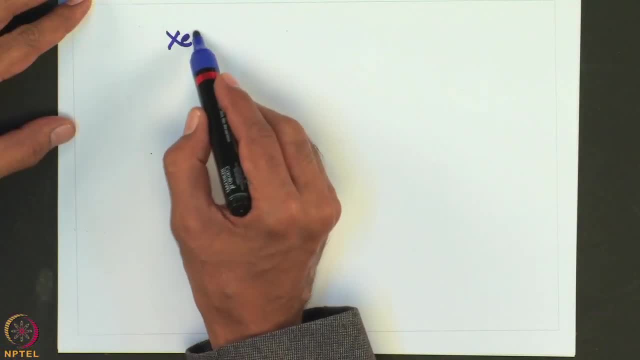 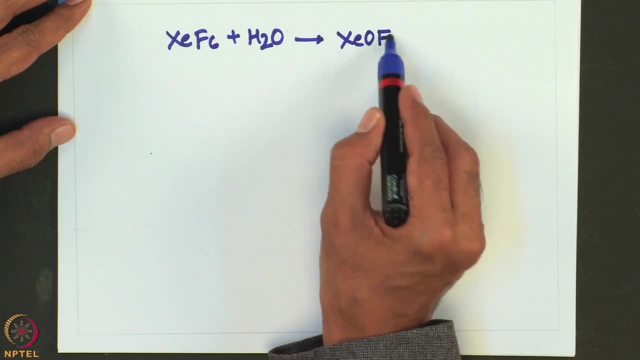 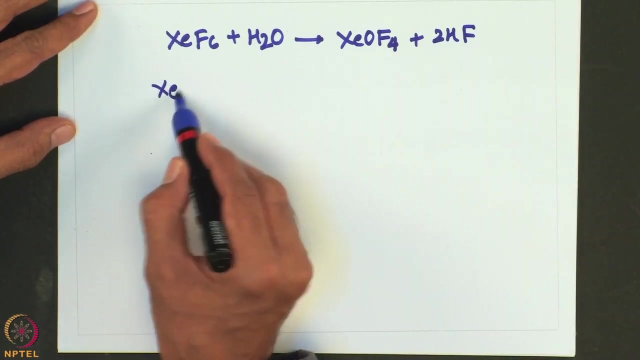 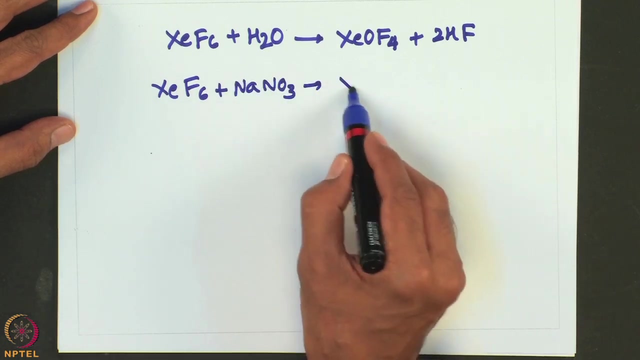 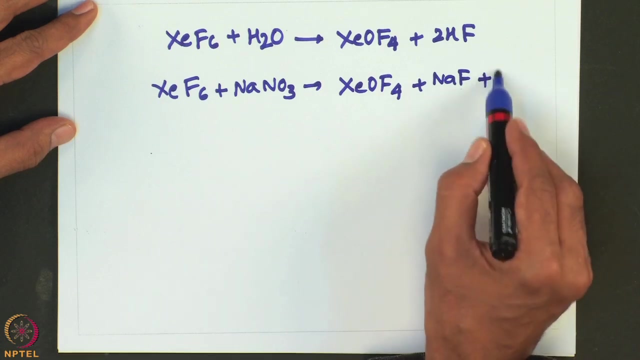 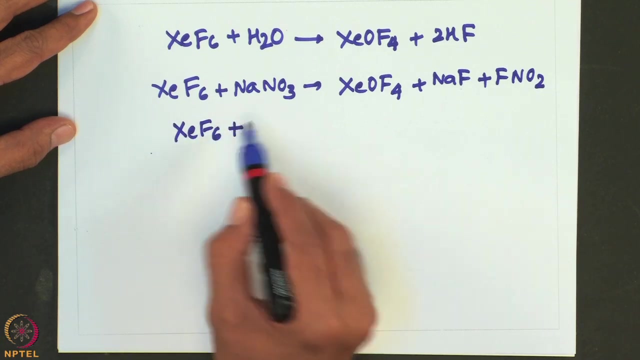 Now, for example, XcF6 plus 1.. Ok water- one equivalent of water- gives XeOF4 plus 2 HF. XeF6 also reacts with sodium nitrate to give xenon oxy fluoride plus NaF plus FnO2. or reaction of XeF6 with phosphorous oxy fluoride. 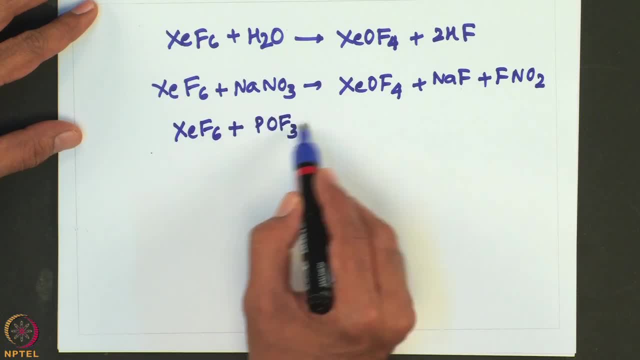 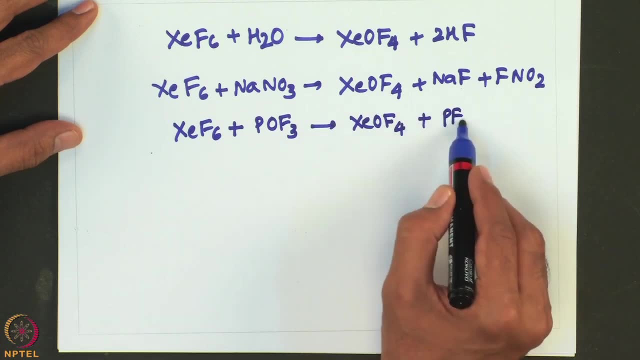 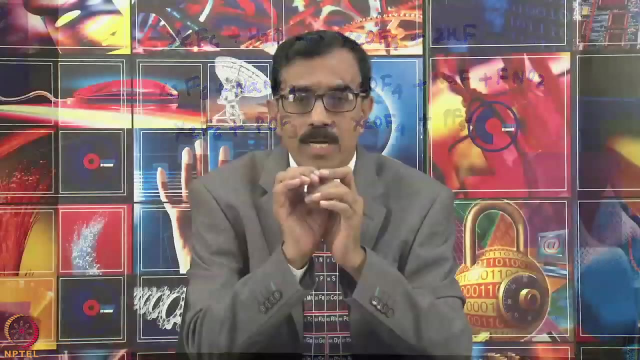 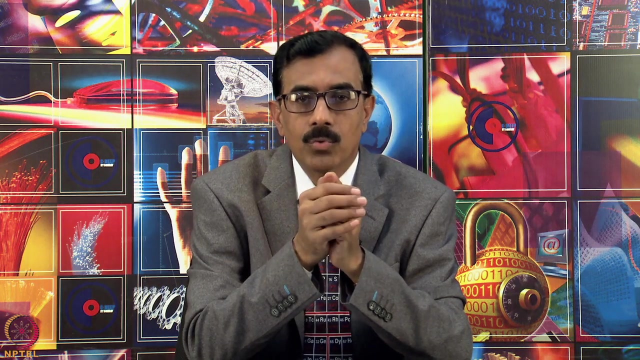 gives XeOF4 plus EF5, phosphorous is getting reduced. reaction of XeF6 with Na4XeO6 gives the oxy fluoride XeOF4 and XeO3F2 and also XeO2F2.. 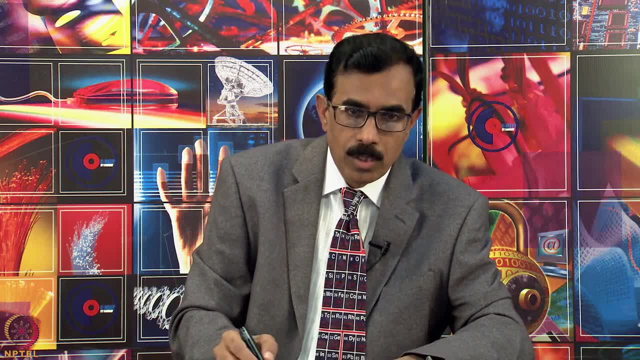 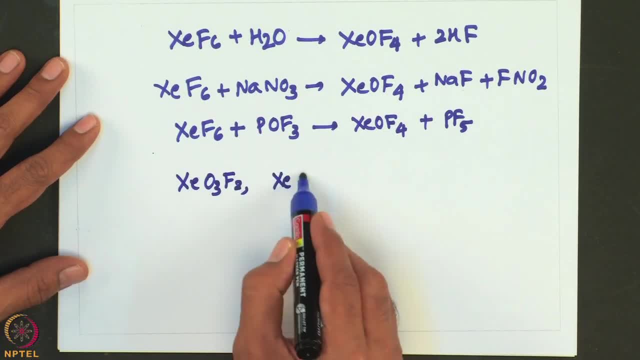 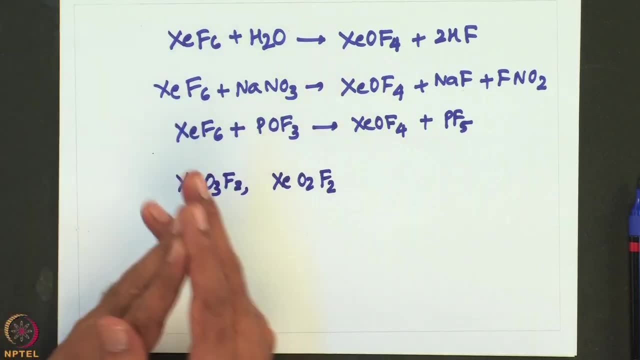 So that means using one of these methods one can also prepare XeO3F2 and XeO2F2.. It is very interesting to look into the structures and geometries and shapes of this molecules. you can try these things at home So other xenon oxygen compounds can be formed from. 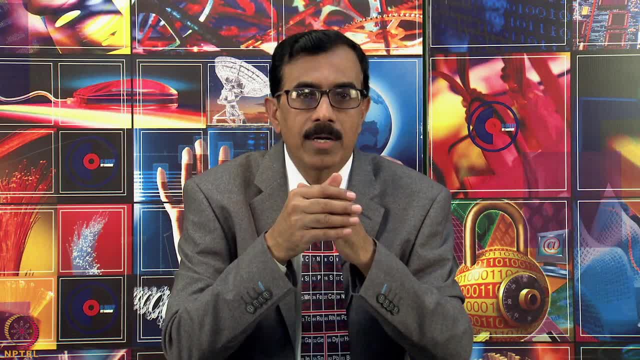 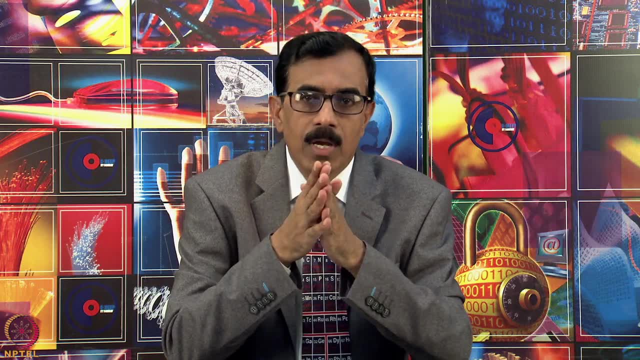 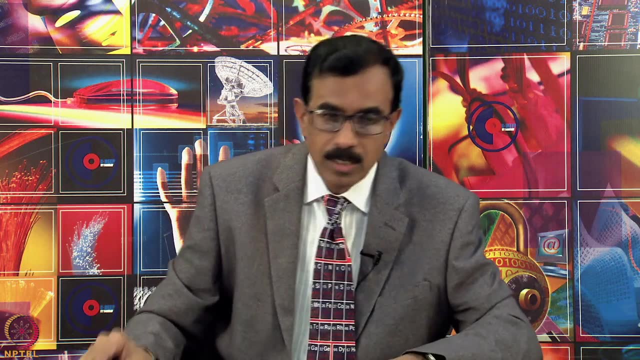 xenon fluoride, xenon tetra fluoride or xenon hexa fluoride by substitution of one or more fluorides by reaction of strong oxy acids such as triflic acid, trifluoromethane, sulfonic acid, with elimination of HF. One example, I will show you So. for example F, XeF with 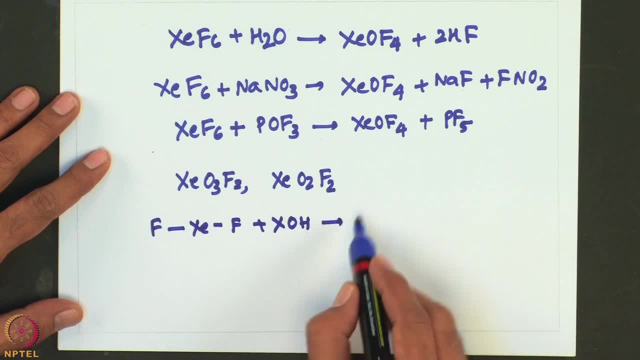 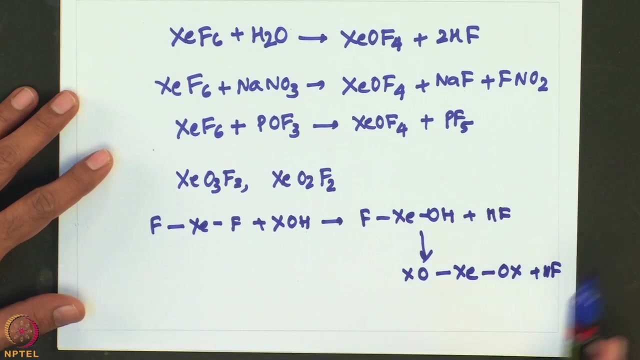 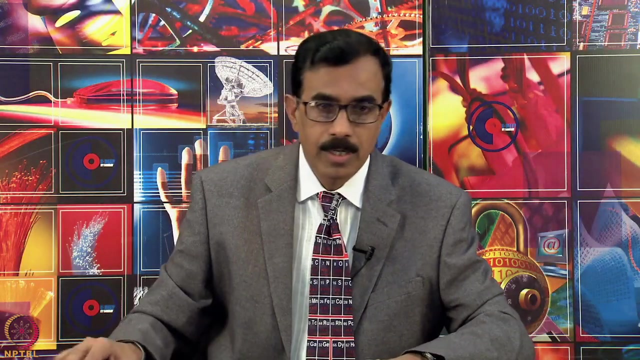 XOH- Ok. Gives F- XeOH plus HF- ok. So of course this can also give XO, XeOX plus HF. Alternately, fluoride exchange yields analogous products. So let me give you a couple of more reactions here. 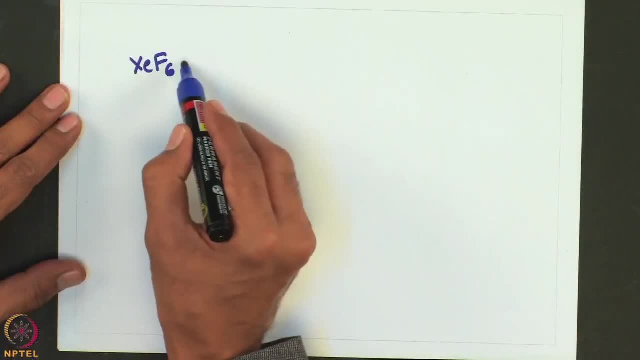 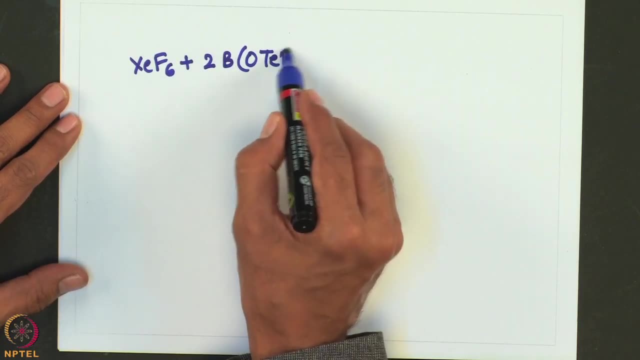 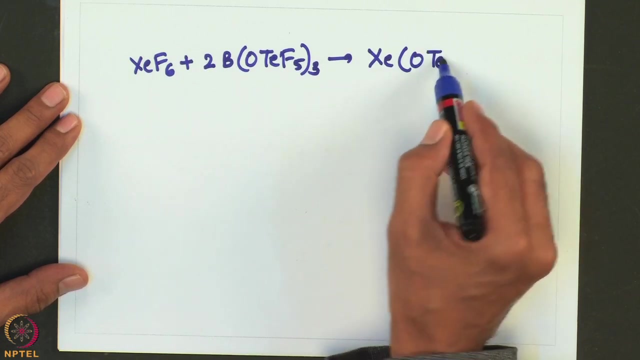 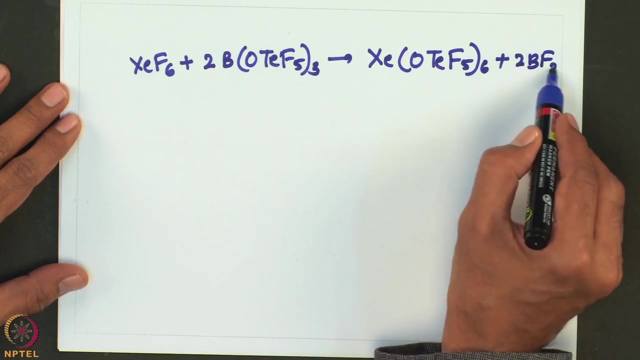 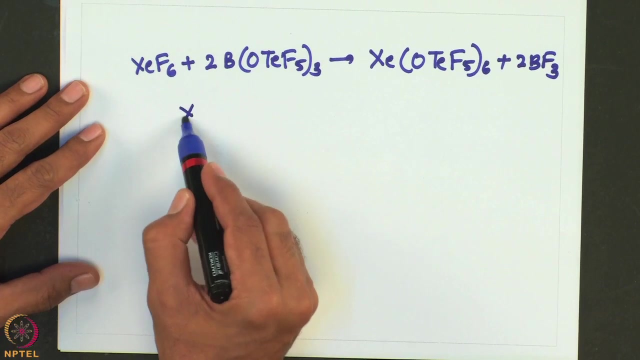 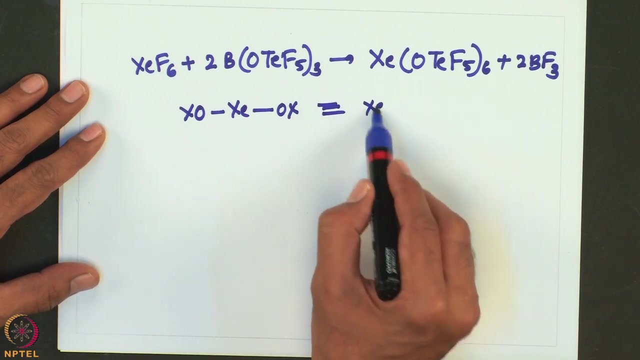 So, for example, XeF6 plus this boron compound, OTeF5. thrice gives OTeF5 6 times plus 2BF3.. So the compounds have similar shapes to the fluorides. Ok, Ok, So if you consider this, XO, XeOX, So this is very similar to XeF2 having linear geometry. 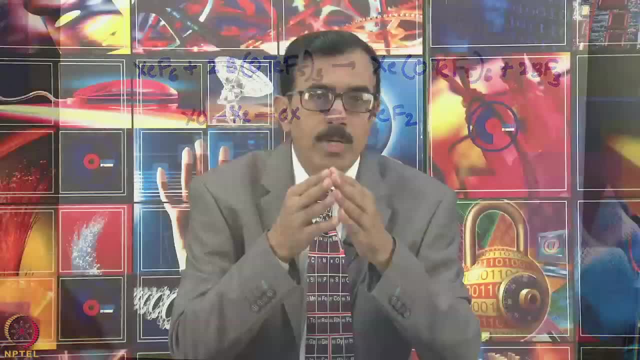 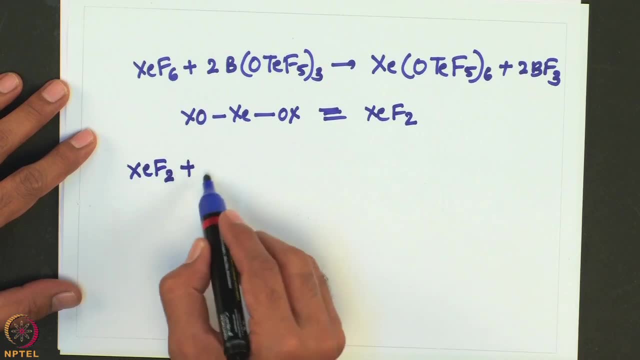 Xenon and krypton. compounds with bonds to elements other than O and F are also known, For example, XeF2. when it is treated with C6F5 3, it gives OTeF5 6 times plus 2BF3.. So 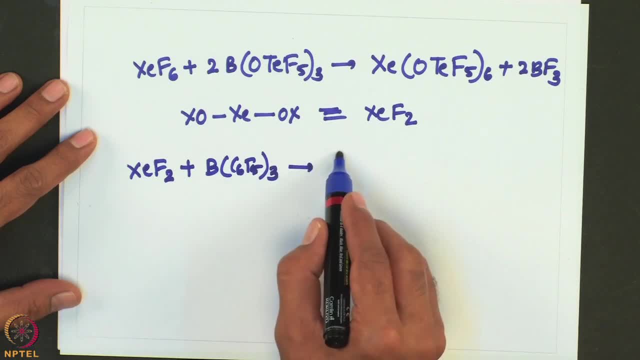 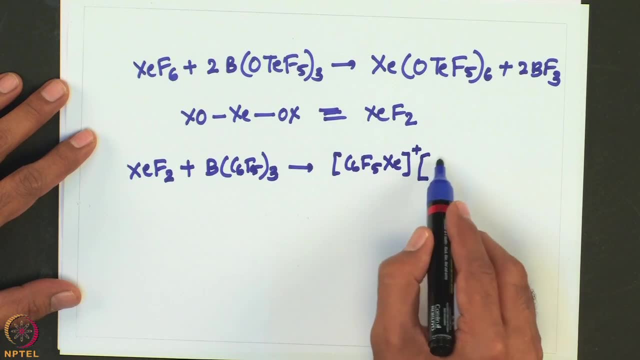 this is very similar to XeF2.. Ok, So if we consider this, C6F5 Xenon plus, C6F5 BF3 minus plus CrF5, C6F5 Xe and C6F5 Xenon, C5BF3, C6C. 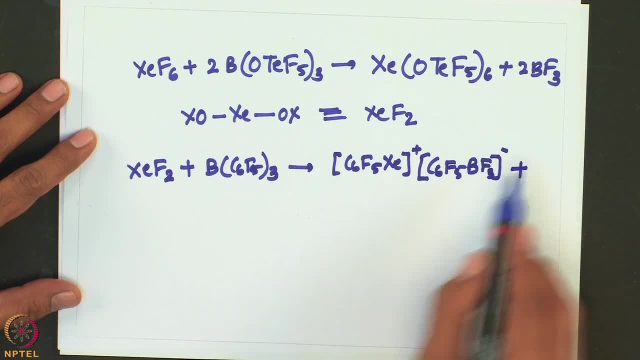 So this is very similar to OTeF5 and Krypton compounds, which gives C6F5 Xenon plus C6CF5 3. So this is very similar to OteF5 Xenon plus C6F5 BF3 minus C6C7 Xenon plus C6F5 Xe and. 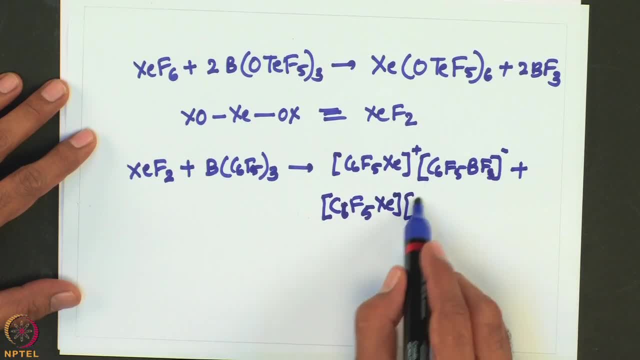 C6C7, Xenon plus C6F5, Xenon plus C6F5 Xe. Ok, Ok, Good, Ok, Ok, Good, Good, Well, do you have any other questions? No, No, Ok, Thank you. 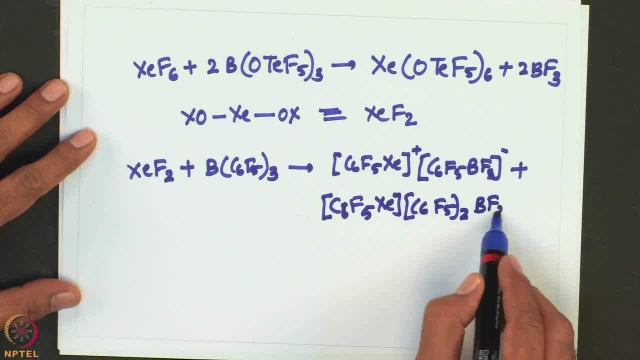 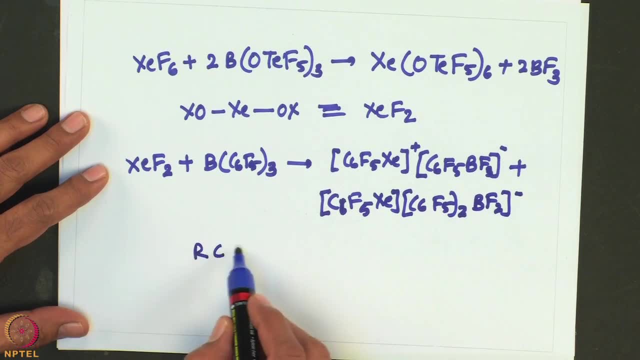 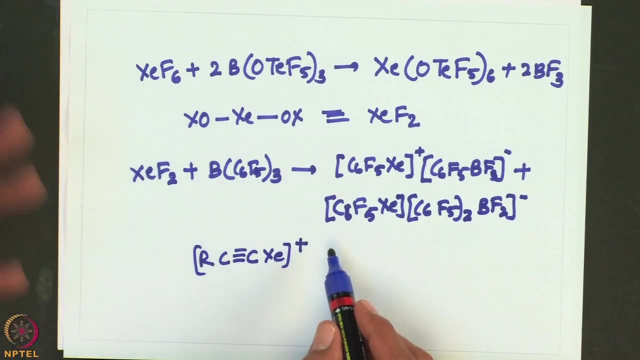 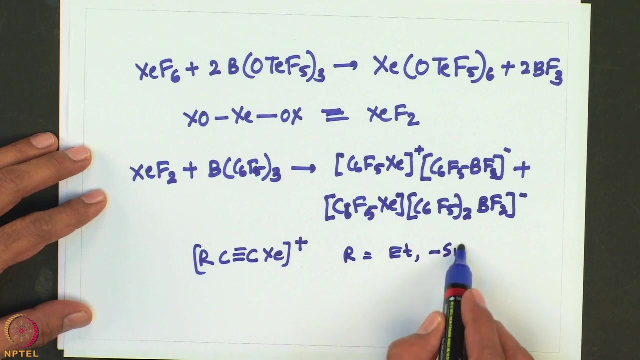 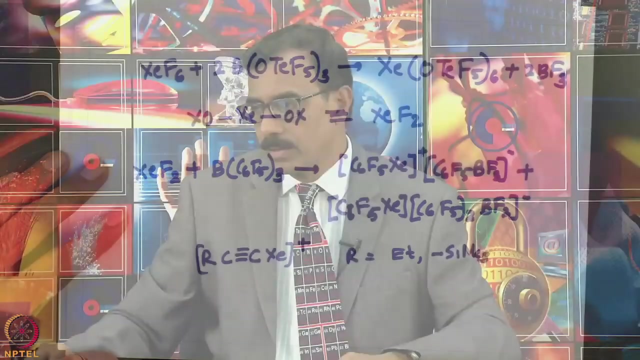 Yes, Thank you. So that means all canal species of the type also known where R can be a range of non-fluidinated groups such as where R can be where ethyl group or SiMe3 group. extensive organic chemistry is avoided with this kind of compounds. 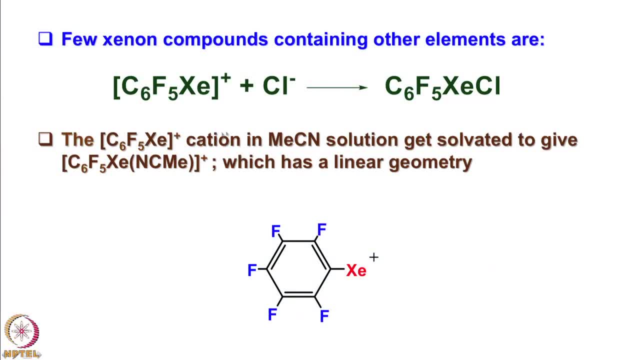 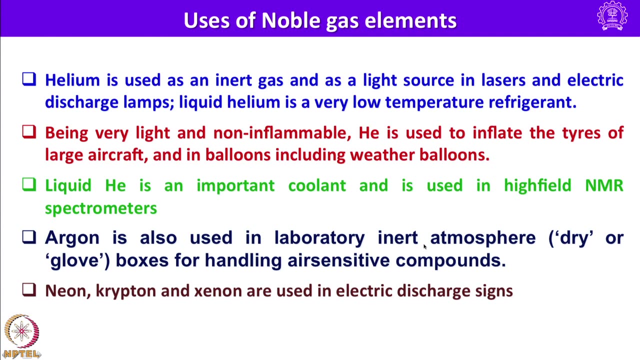 So you can see here in this slide how this compound reacts with chloride to form a neutral compound, and also one can also see the formation of xenon to carbon bond here in this one pentafluorophenyl derivative. ok, So let me talk about the uses of noble gas elements before I summarize.